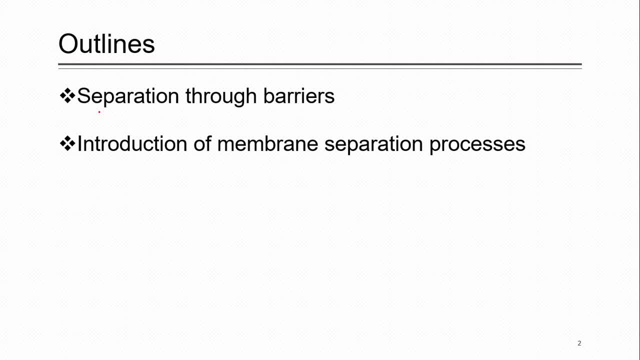 So in today's lecture we will start from very basic stuff, that was separation through barriers. so I will just go back to the lecture one and two when we started this Subject in the start of semester, and I will mean recall few things from there. And then we have to jump towards membrane separation processes. 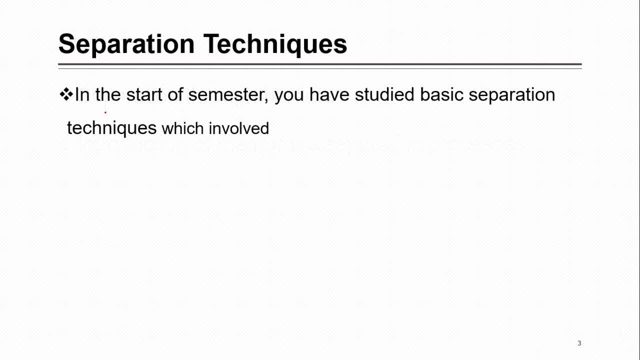 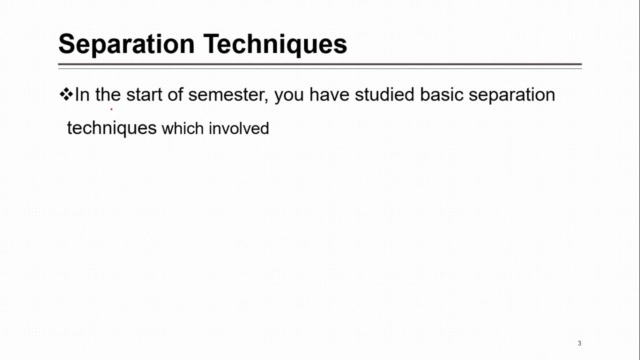 So let's start with this. So, as I said in the start of semester, you have mean studied Some basic separation techniques, that actually, when you go for separation, They can be classified or they can be categorized into four separate categories Or four separate techniques, and mean, when you talk, 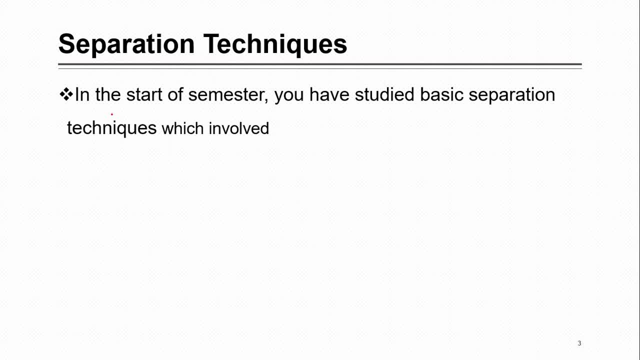 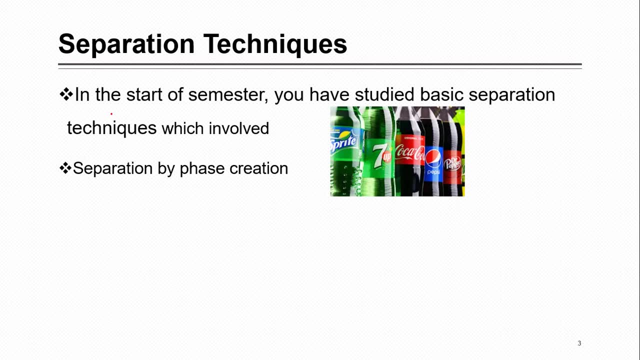 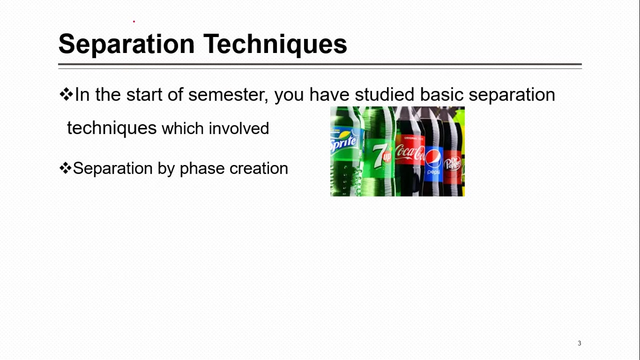 Generally about them. you can classify them in four categories and those categories Involved first one was separation by phase creation. and in separation by phase creation, This means that you have to create a new phase That Provides you separation of one component from the other. for example, here you can see these cold drinks in. 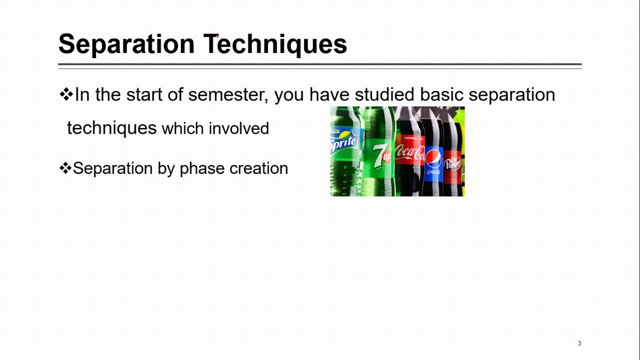 These- I mean this is very common example, Which you know, which we have also discussed in this- what happens when you open the main, this bottle? Actually, you release the pressure, you reduce the pressure and, due to reduction in this pressure, Gas, co2 is evolved from this liquid. co2 is actually filled with the pressure inside liquid and when you will open it, 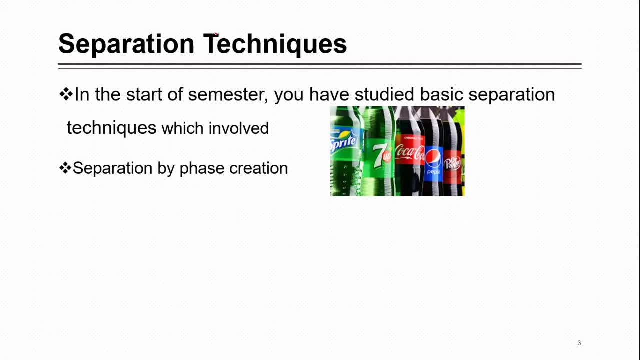 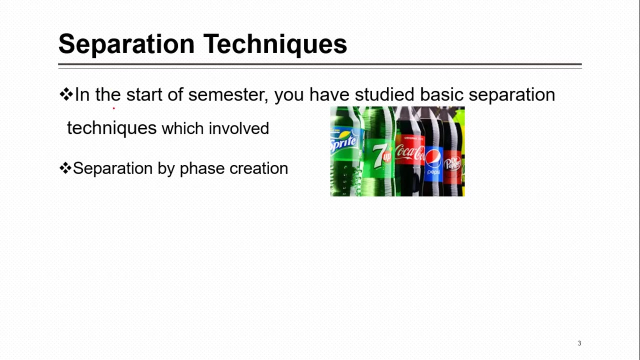 Due to this change in the condition, due to this change in pressure, This gas evolve and that's formation of a new phase. That's that was dissolved here in the liquid but now that is released in the form of gas. This was phase creation and Related to this you have discussed or you know. the technique commonly used in the industry is distillation, in which you provide a 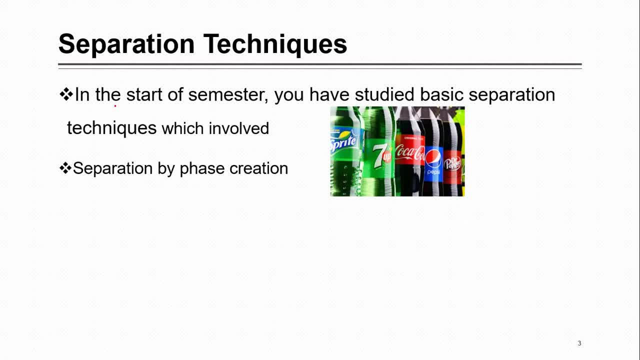 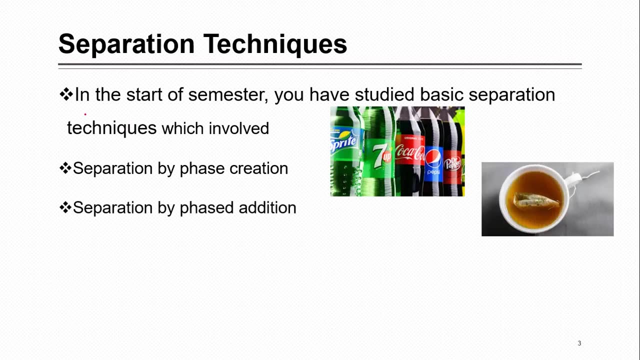 high temperature, and with the help of that you mean vaporize some part of your feet, while other is in the form of Liquid, and they get separated. So here, when you are vaporizing something, you are creating a new phase. So Next is separation by phase addition. 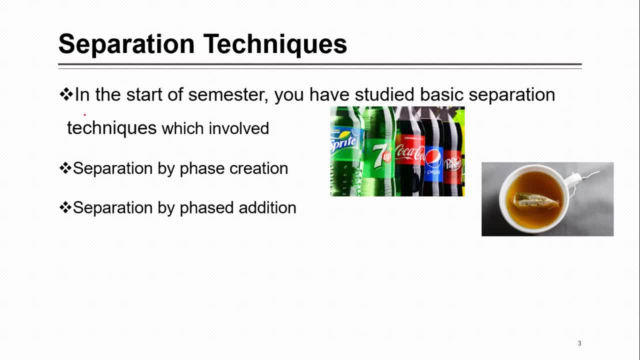 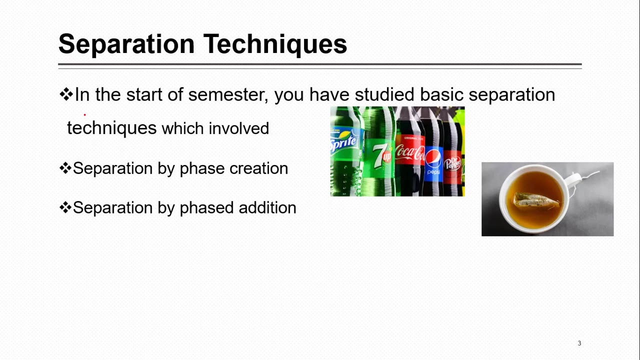 Separation by phase addition: here you will separate something by adding a new phase. for example, here very common example or simple example you can see- is like when we add hot water to the Mean, this tea beads or tea leaves. So what happens? some something is extracted from this solid beads towards water and 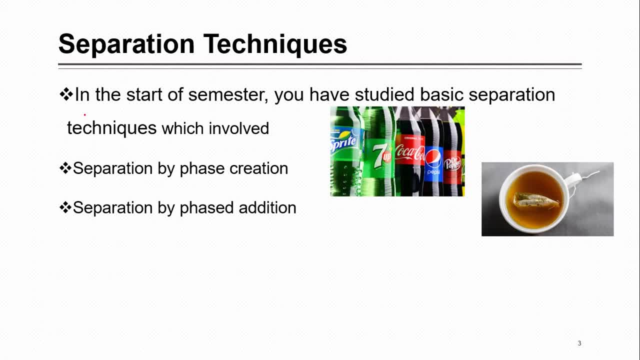 in. Similarly, there are some other techniques on industrial scale which you have discussed, and they involved actually Absorption in absorption- you remember that we discussed the topic in detail and you always introduce some solvent for removal of some components from the feed. and then, after this, we discussed 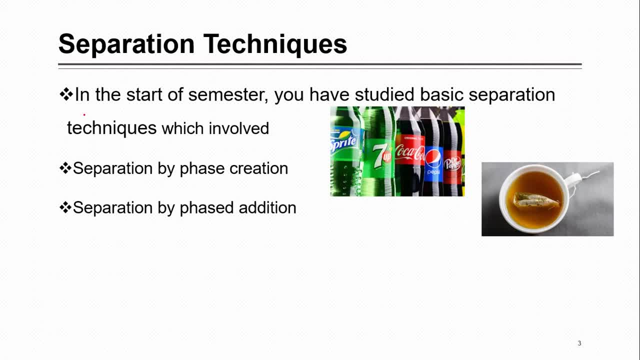 I mean, in last few weeks, liquid, liquid extraction. So what we were doing there, we were introducing some new liquid and that was like phase new, phase addition and with the help of that, We are separating some components of our feed That was solute, which you were, I mean. 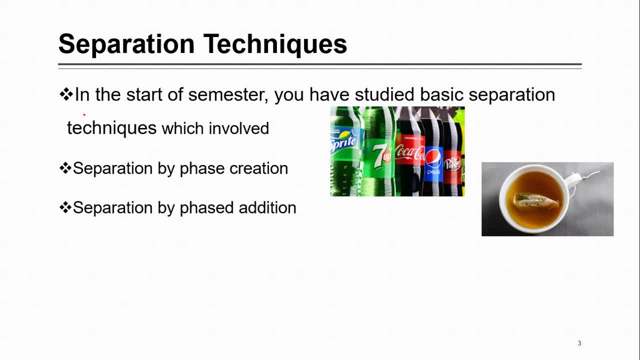 extracting with the help of externally introduced solvent as well, one technique which still we have to discuss at the end of this semester, and that's leaching solid liquid extraction. and this example of T is actually that solid liquid extraction, because we are extracting something from the solid that is beat with the help of some. 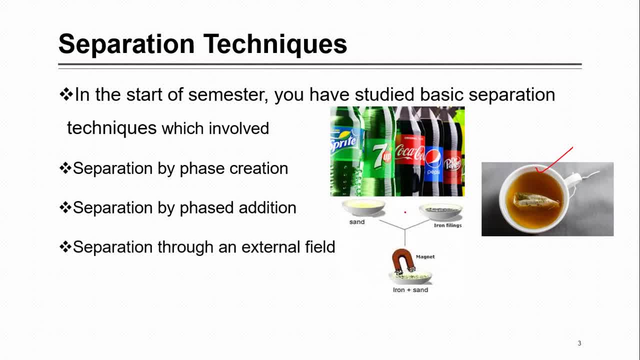 liquid and Then there is a pressure through external field, in which you apply some external field and you get separated some mixture. So in this example, Which you commonly know from the FSC class there, this being used here and And some technique which on industrial scale is used, called electrophoresis, I think we 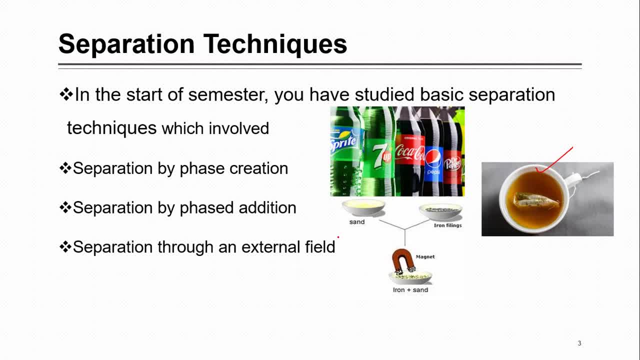 discussed in the start of semester, which is usually used in some how nuclear industry, I think, and they are used. they are externally introducing some fields. So here externally introduced field is magnetic field and with the help of this you can just separate iron fillings from sand. 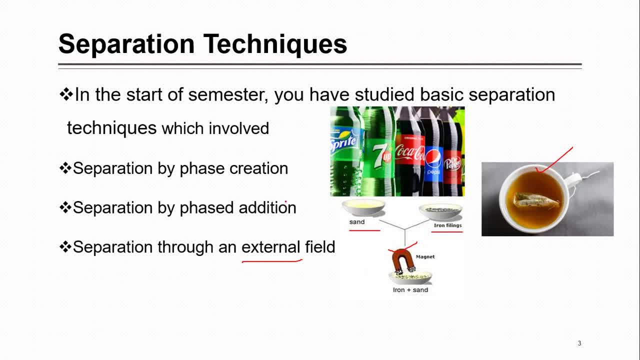 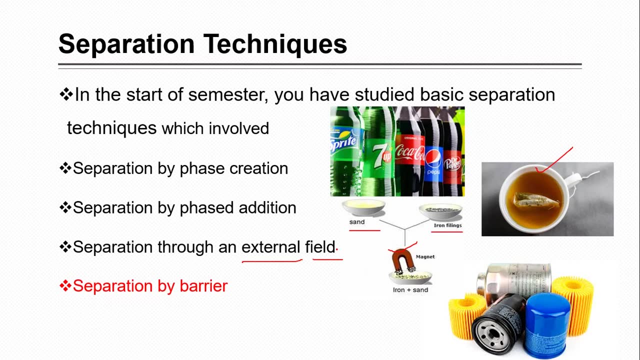 So here you did not add any like new phase, you did not created any phase. but what you did? you applied any external field, external force, and with the help of that you have separated a mixture. And then there was last type four technique, or fourth category, and that was called separation. 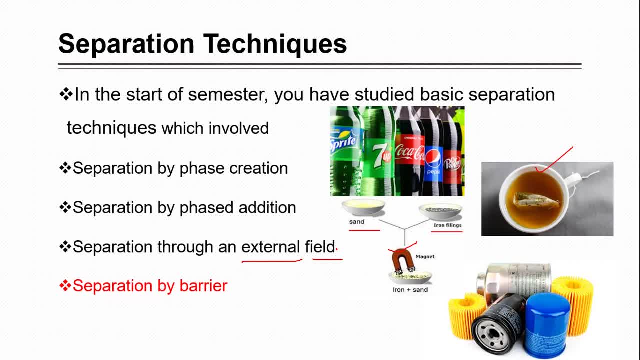 by barrier, or you can call it separation through barrier. In that we discussed various example I have in the next slide. So here you can see these are called filters. Some are air filter while other are oil filters. we discussed this example there. So in this what happens actually? you are separating some components from the others with the help. 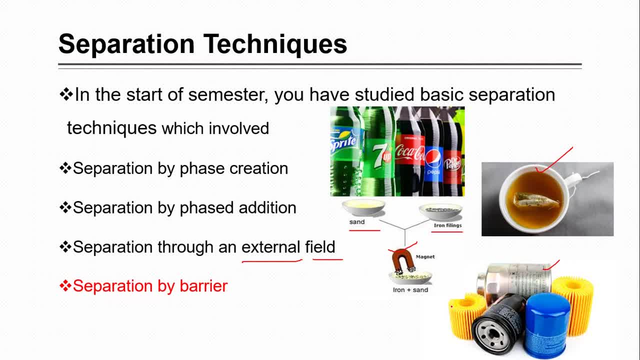 of some barrier. For example, if you talk about air filter, what happens? air which is going to enter to your system, to the engine. So that is mean we just purify that air, we remove some dust particle. other means some also, something like if there are some particles which can go to engine and can 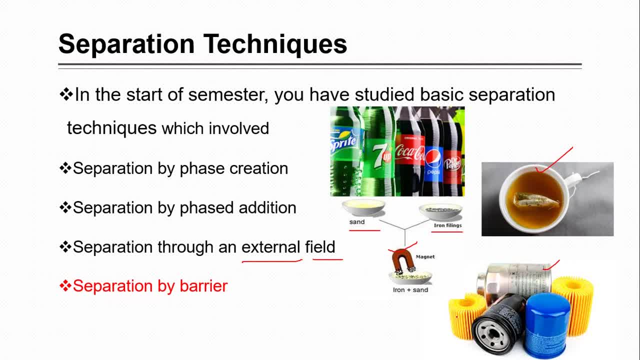 damage that they are removed with the help of this filter. so when air will pass through, air will go through, but those solid particle are trapped inside this barrier as well. if you look at these oil filters- so oil filters- we remove some solid particle present in the oil so it didn't damage the parts of 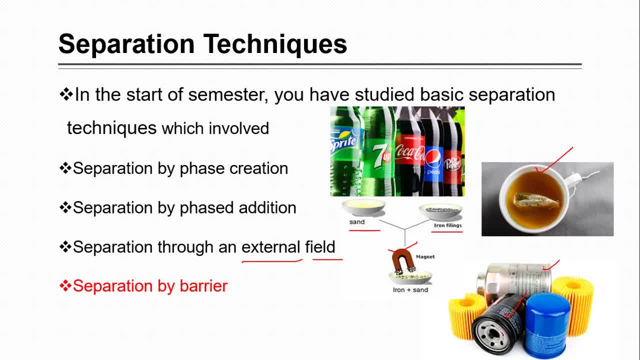 engine through which this oil is being circulated. so when you will pass that oil through this, these oil filter contains such structure inside that that will allow only oil to pass through, while if there are some solid of some specific size, they will be trapped inside this filter. so in clean oil will. 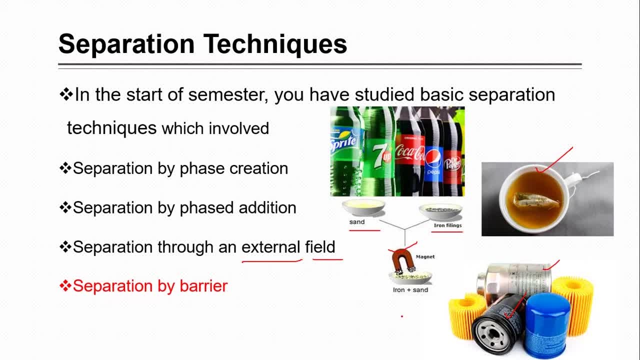 be moving towards your moving parts. so we have to actually take this separation by barrier and discuss in detail. so, through separation through barrier. yes, before that I jump to what next slide. so if I talk about the industrial example, about this, so that's membrane application, and there are various type of membrane application which come under 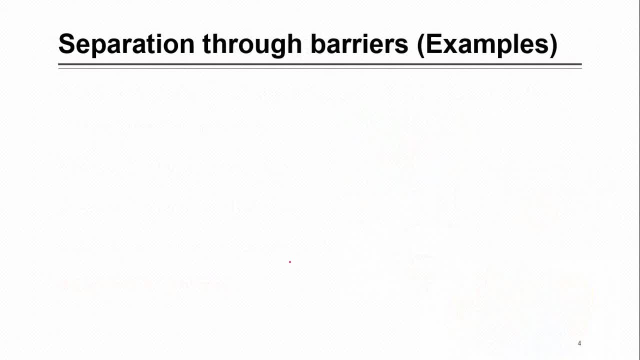 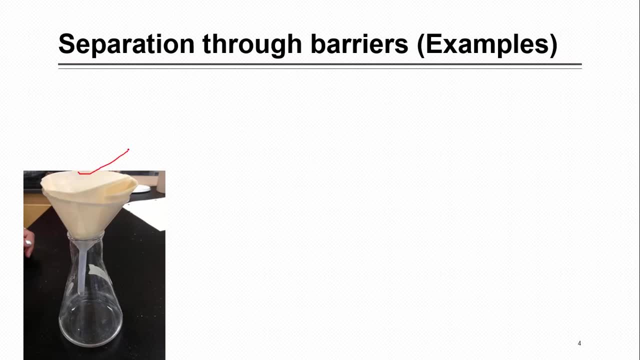 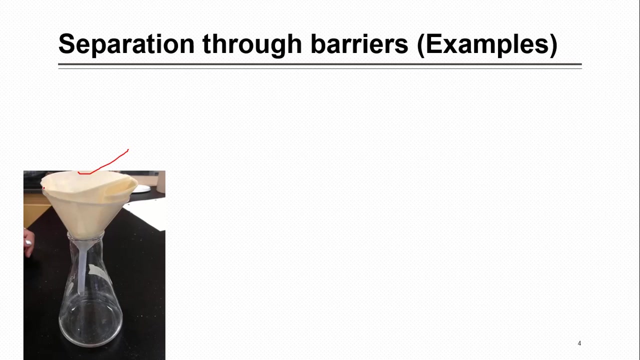 the category of separation by barrier. so there were few common example which were discussed in the start. so you can see here this example which you commonly use in lab mean: when you are separating some solid you go for crystallization and for various analysis in chemistry when you go through this. so here what we do: we will just pass in the liquid. 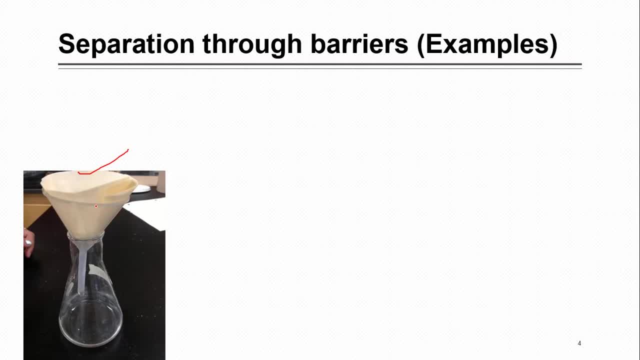 and solid. so I can say: mixture through this. so when it will pass through this, you know that solids are retained on the surface and liquid will pass through. so this is just separation through barrier. we didn't introduce any news in phase. we didn't create any phase. what we did. we didn't apply any external force here, at least in this. 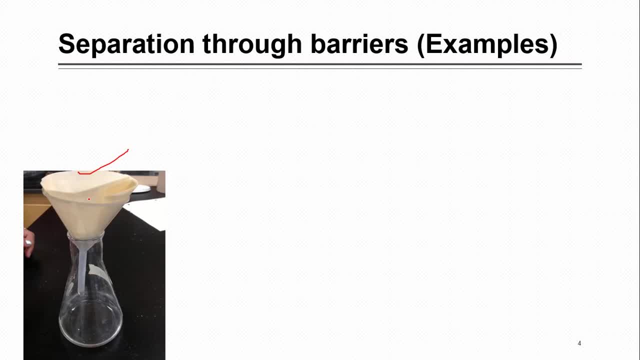 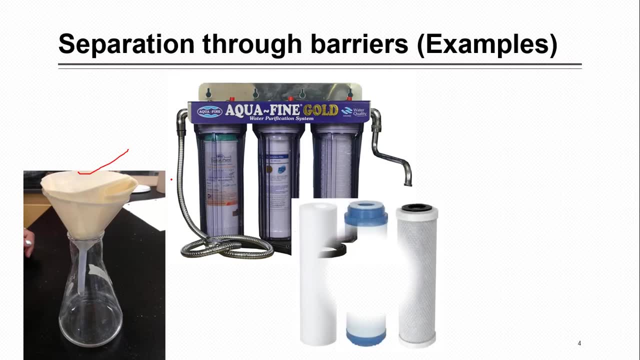 case. So what you did? you just provided one barrier and separation takes place. Then these water filters: you commonly know that they are used and here they actually contain some. the filters of various sizes are various material actually, and they capture the solids of various sizes through the water So that we can we can get, at the end, clean water. So this is. 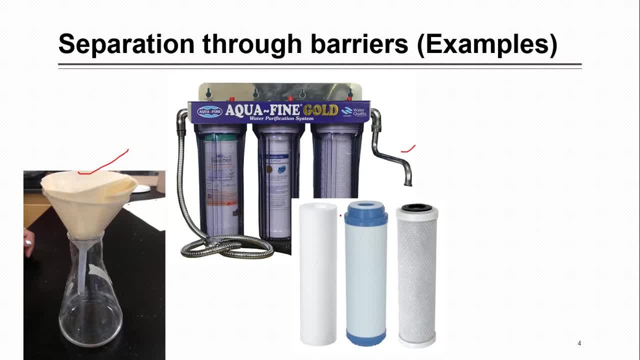 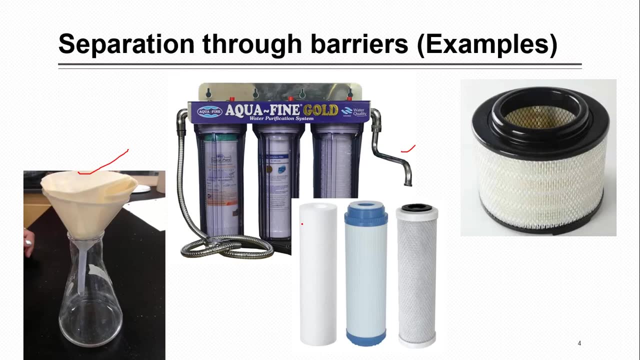 again the separation through barrier, in which you are applying one barrier which is a filter and based on particle size, it is making separation, And then this is, I think, air filter. So in this, when you pass air through, this air will just get separated because air will pass through. 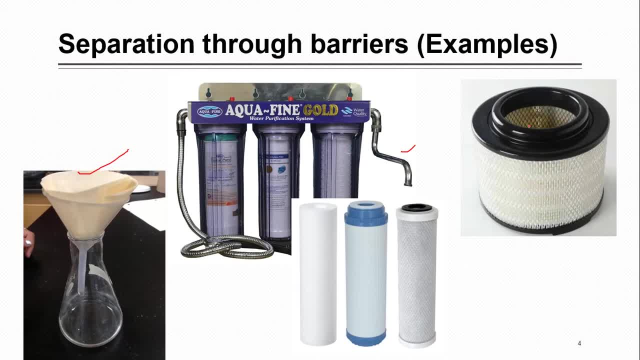 but the solid particles are untrained on the surface. of this either I mean inside or outside. I mean it will depend on the direction of the flow, from where you are flowing this air to, in which direction, Suppose I am, just air is entering from inside and leaving, or 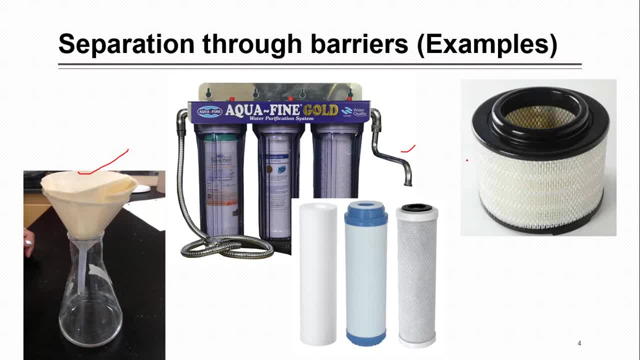 pushed outside, So all those particles will be entrained inside. and if you are pushing air from outside towards inside, So here then solid particle will be, I mean, entrained on its surface. So all these are example of separation through barrier, but they are being used on small scale. So if we have to talk about on large, 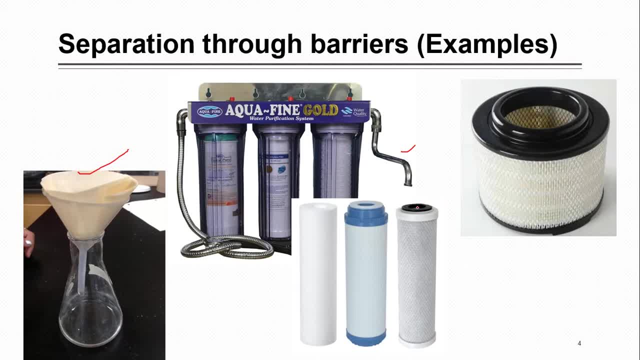 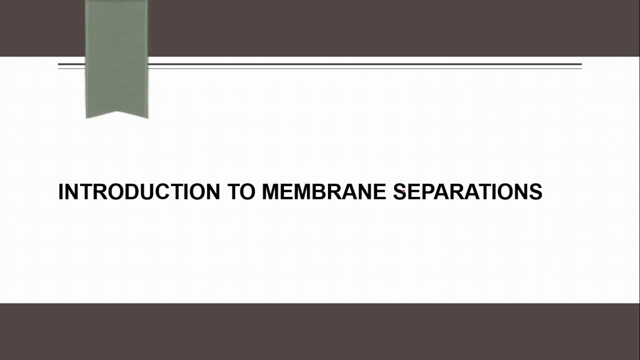 scale, industrial scale. So then there is example of actually membranes, that is, I mean separation through a barrier. membrane can be considered as a barrier which will allow the separation of various components of the feed. So let us look at this. I mean membrane separation, Like when we say membranes, I mean membranes. 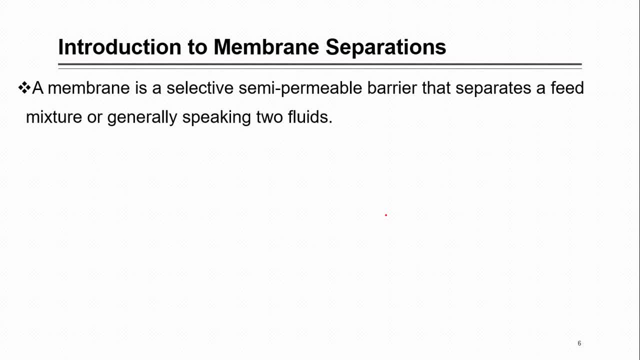 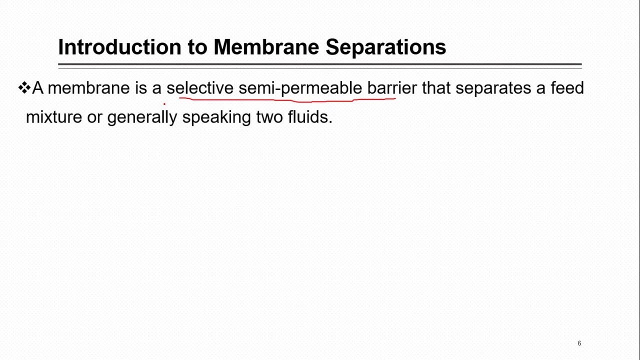 as I said in last slide, that this is separation through some barrier. So that barrier is working in such a way that it is selective towards some components, or it is like selective semi-permeable barriers. So membrane actually can be defined as selective, semi-permeable. 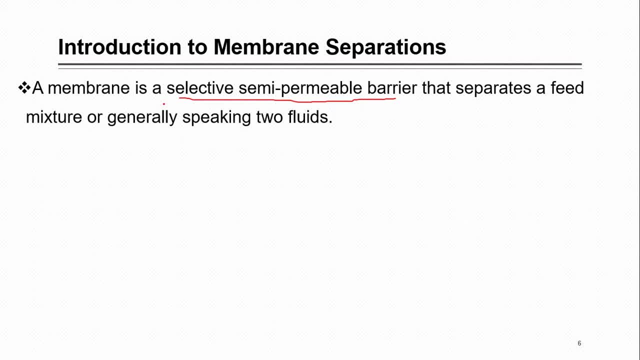 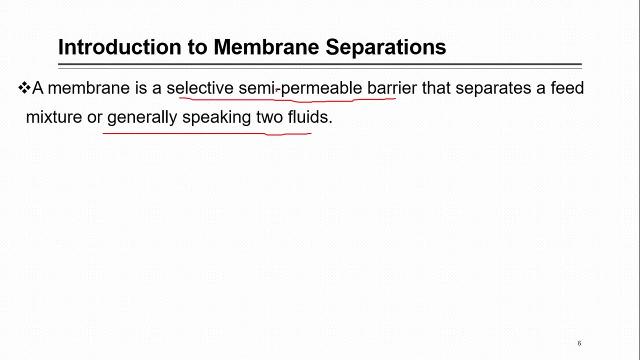 barrier that separates a feed mixture, I mean into its component, or you can say, generally speaking, if I just say there are only 2 fluids inside my feed, So membrane is a semi-permeable, permeable barrier that will separate two fluids into two streams. So this semi permeable- 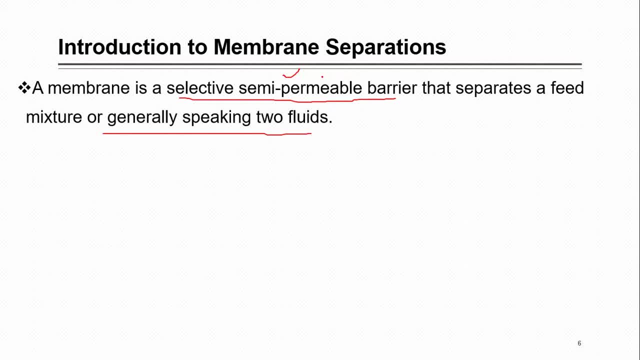 something which is like selective for some components, which allow some components to pass through while other will be retained on its surface. So this you can compare now with those which we have just discussed, that they were also allowing some of the component to pass through while others were retained. For example, water filter that allows only 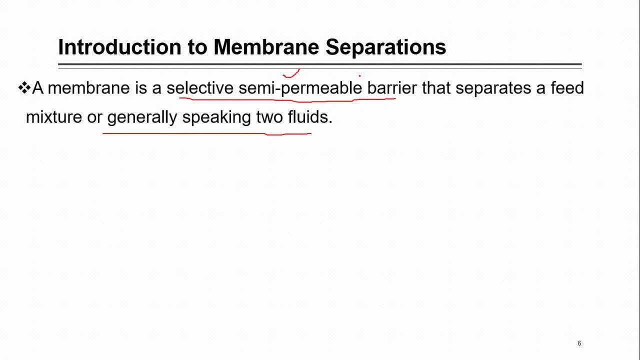 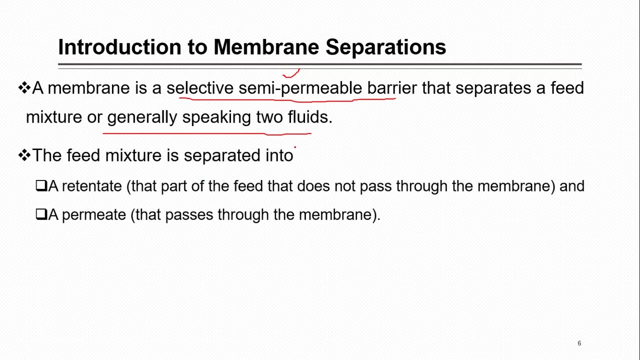 water to pass through, while other solids or some impurities present in that water are just, I mean, retained on the surface of filters. So here the same methodology will be applied. So overall, when we say that, I mean feed in the gas is separated into two parts, like actually. 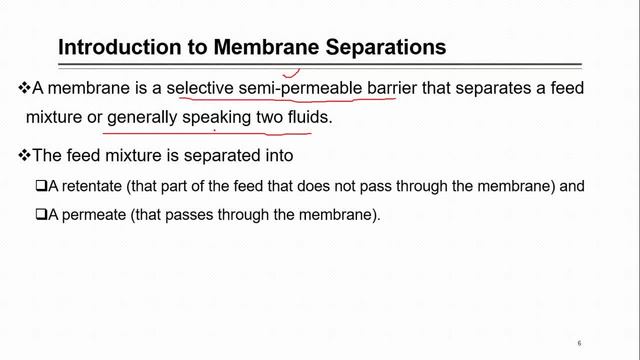 one part will. one part will pass through the membrane while other part will be retained on the surface of membrane. So they are given some specific names in the filter, So the name is few names. like one part will be retained on the surface of. 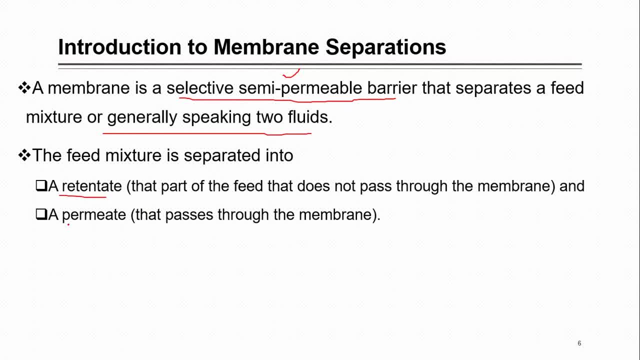 membrane. So they are given some specific names in the filter. So they are given some field of membrane separation. So they are called actually retentate and permeate. Retentate is that part of the feed that does not pass through the membrane is named as retentate. 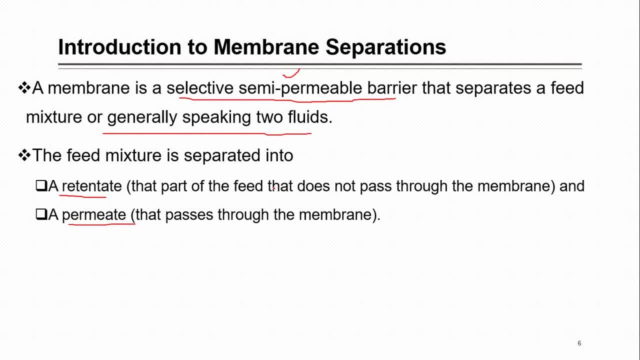 something which is left over, which is not allowed to pass through, is called retentate and while there is something called permeate. So permeate is that passes through the membrane. if you look at the meaning of this word, permeate- pass through- that will. something will pass. 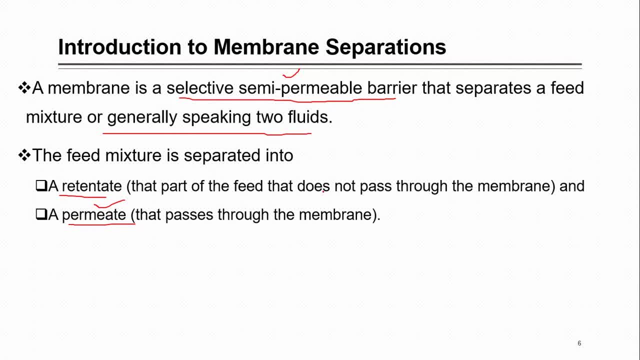 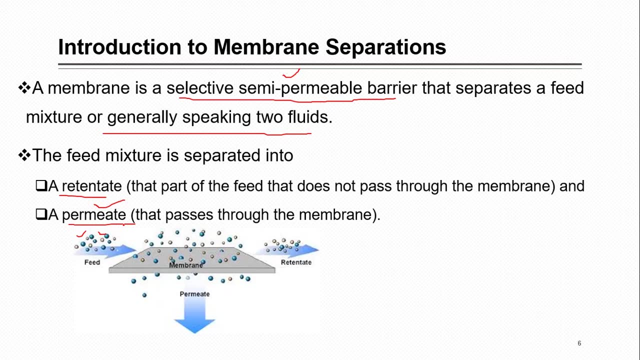 through the membrane that will be called as permeate, So when our feed will be entering to this system, for example. here you can see that we have a feed and that is a mixture of, like here, two components. it is not necessary, sometimes we can have more than two components, So our membrane will be selective for some of. 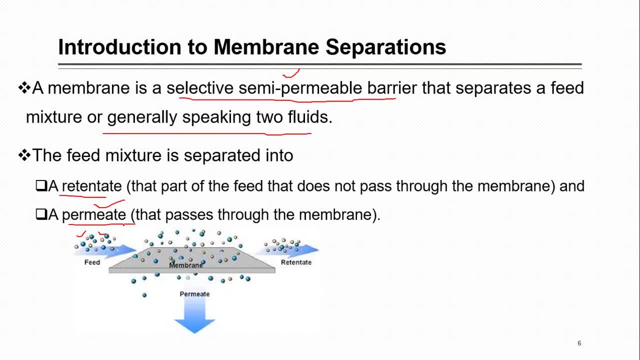 those and we have to select such membrane that it means it gives us separation. For example, here means two fluids are present and in this feed, when you bring in contact with the membrane, So through this membrane, some of those will pass through. for example, this is selective. 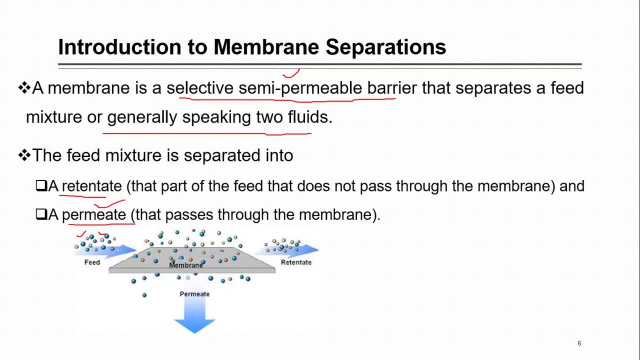 more selective towards. like these blue colours I mean chemical or you can say blue colour component. So those will pass through this membrane, while other, which are retained on its surface, they are called retentate, So they will just leave from here as such. 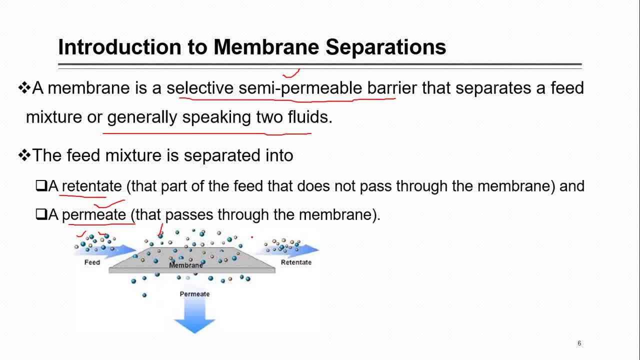 So overall, one thing: you can observe even from this figure that this is not like 100 percent selective toward one component as well. one of the component which we want to completely separate is not being done here overall, because you can see in retentate some. 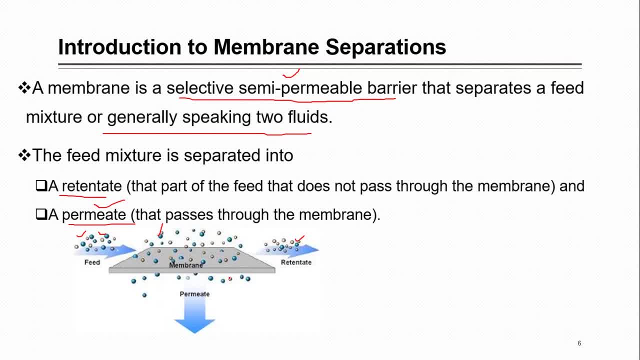 of blue, I mean component- are present, while other, silver, some are. some has passed through this. So actually, when we will talk about the various membrane, their- I mean construction material of, I mean material of which membranes are actually synthetic. So you will see that we have to look for something called selectivity. 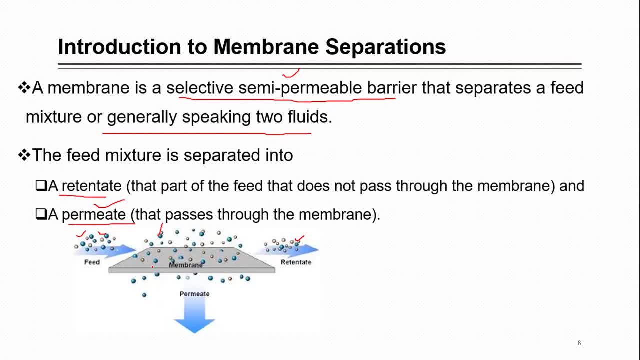 So here I mean its selectivity. I mean this membrane is highly selective for one of the component, but it also some other will also pass through. this, I mean overall may be another question can raise in your mind here, because if we see these blue colour component as he 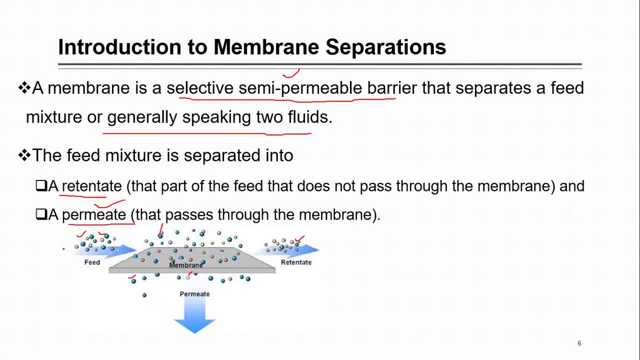 has shown here. they are large in size, while other silver one are. I mean, some are in size. So in this case, if it is separating based on particle size overall, what you will see, that definitely something I mean which is small in size should have passed through this. 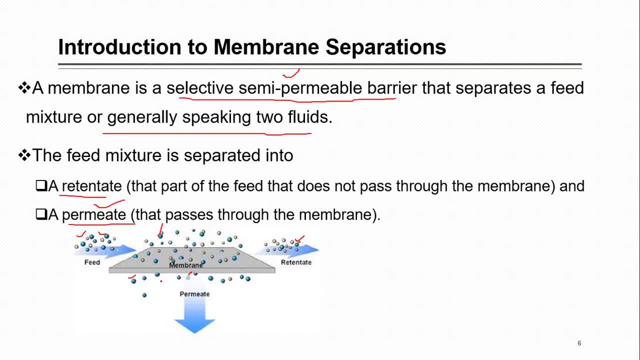 while other should stay on the surface, which are large in size, but here opposite is happening. but actually these membranes are more than just size separation. some other phenomena also involve here, So which we will discuss later on. So overall, just remember here up to here that these membranes are selective for some. 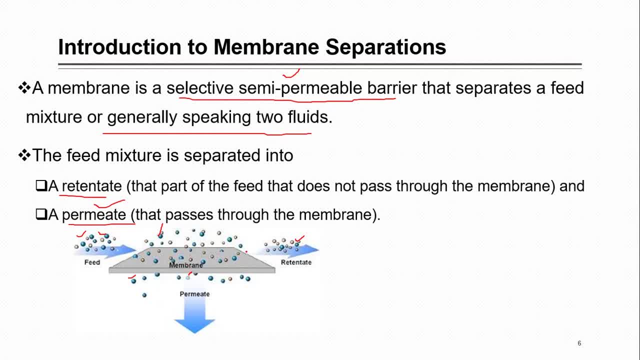 component. they allow some of the component to pass through, while others did not pass through. this And one thing here. actually, this will also differentiate it from the filters. filters which we use, they just are working based on size. I mean any component which is large in. 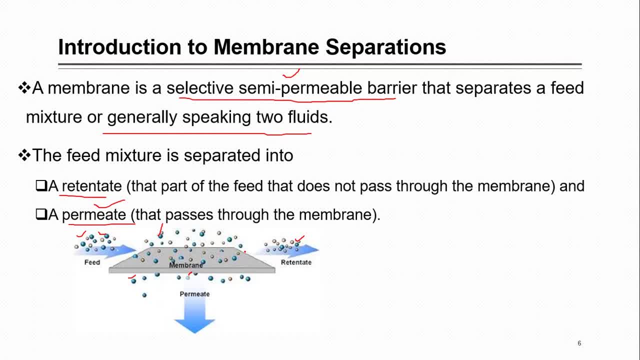 size will be retained on their surface and small will pass through. So here some other phenomena will also involve so that differentiate actually these membrane from common simple filters. So overall here I mean this is This schematic from your text book so that presents like your feed is entering to the 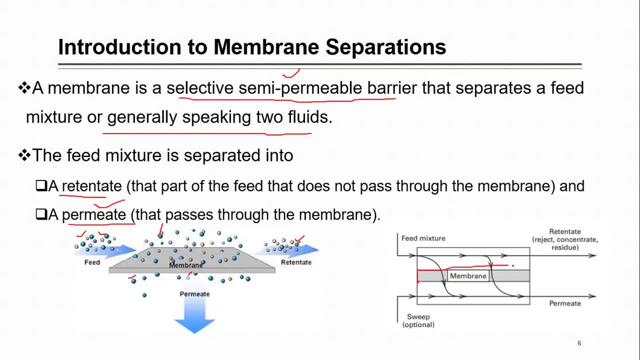 system and then there is a membrane. this barrier, which is a membrane- So this is some module- through this feed is entering from one end and it is leaving on the other end. So overall, through this module, we can see that, like this, some of the component is just 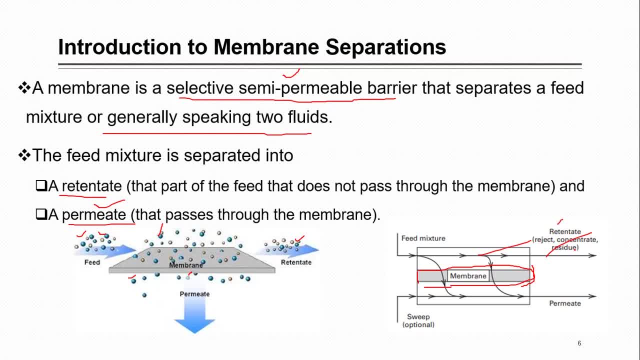 passing through and that is retented like rejected, something which is not passed through the membrane, While other which will just pass through. So some of the component will pass through this and that is called permeate. So here he has indicated something sweep. I mean. this is to, for example, sometime you 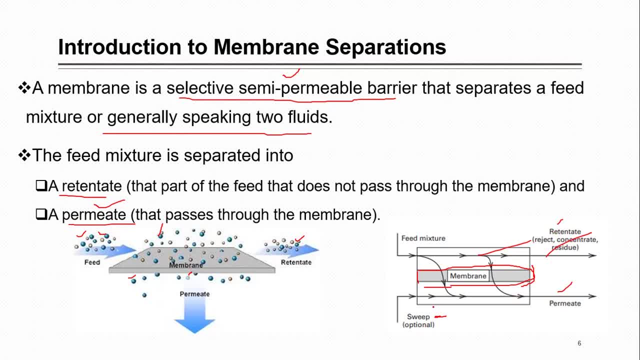 have to remove the permeate from the system So you can remove with the help of some external aid So it did not accumulate here in the system. and like sweep this word- you know that when you just pass something to or you remove with the help of something. 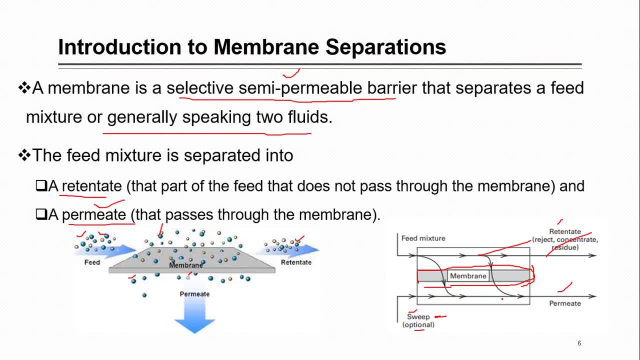 So just this is optional Sometime. So some system actually we have to remove from our system, from our assembly, the permeate that it did not accumulate as well. its- I mean- passage is easy through the system, So you can sweep with the help of some external aid, for example if there is some gas being. 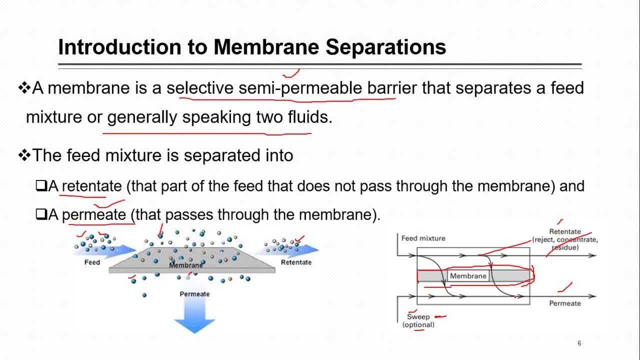 accumulated here. So maybe I can bring some of the gas, of similar gas which is highly purified, So I can push with the help of that, or sometime, if it is liquid, So we can also, I mean, bring from here some pressurized liquid. 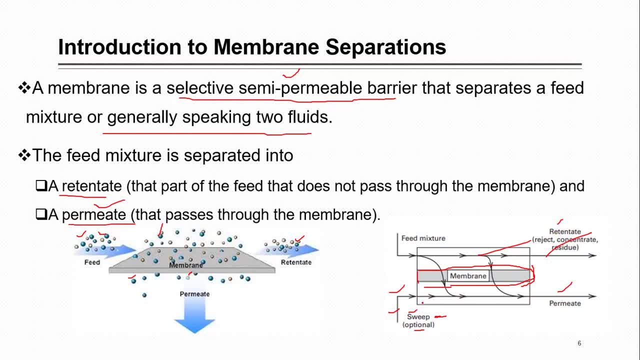 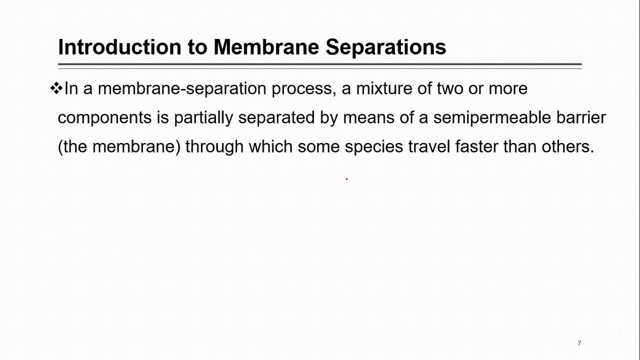 So that can help as a sweep that will help us. I mean, with the help of this pressure your permeate will leave from this system. So overall, when you go through the membranes, what they do actually membrane separation. this separate actually mixture of two or more. 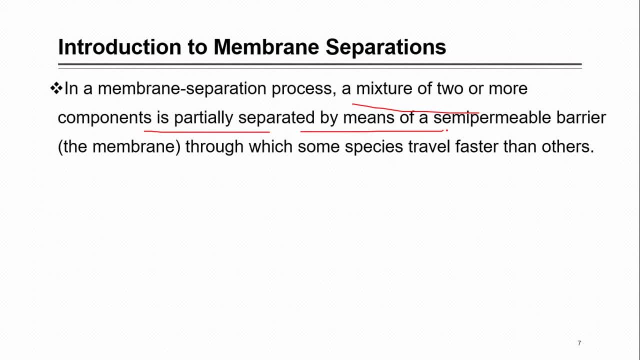 component, So that partially separated by the means of semi permeable- Sh 역시 꾸- receptor membrane, or a membrane through which some species travel faster than other, As I have mean told you in the last slide, that you see here mean it is not only 2 components. 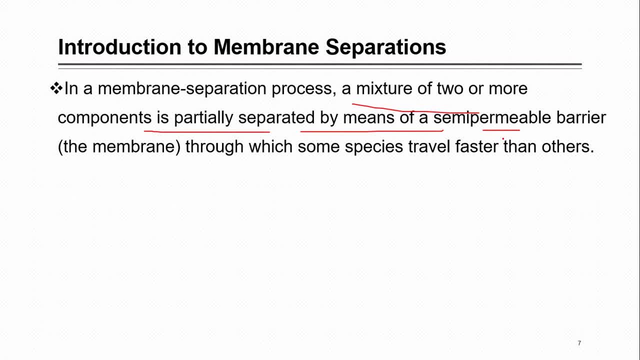 sometime in the field there can be more than 2 component. but here our purpose will be to separate 1 or 2 of those. it will depend on the application. we will look So there can be sometime more than 1 or 2 component. for example, if I give you the example, these: 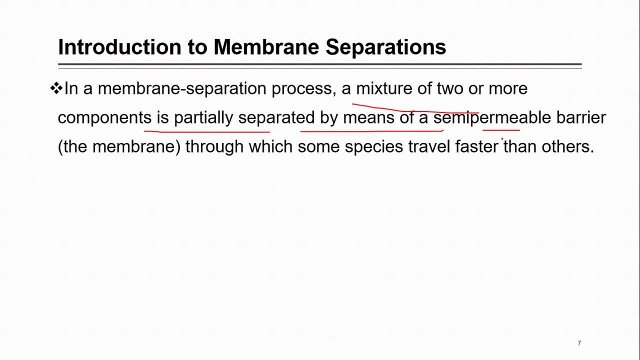 membrane are also used for purification of water, like in the start, some somehow we talked about this, like desalination is one of the technique in which would you do? you just purify the sea water with the help of membrane. that is called desalination. 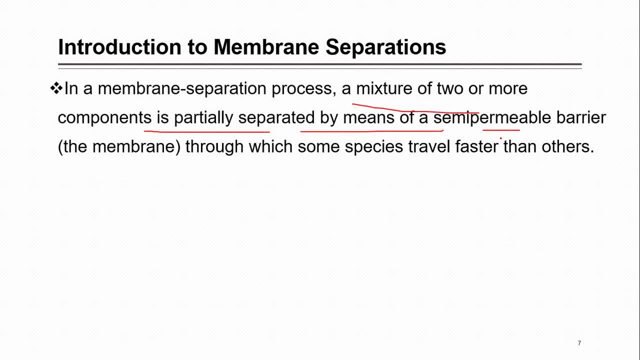 So in that case mean, as you know, that if you take the sea water that contains water and hundreds of other mean impurities. So although we remove some of those before bringing it to the membrane, But still when you will bring it to the membrane, that will be not only water and 1 of the component. 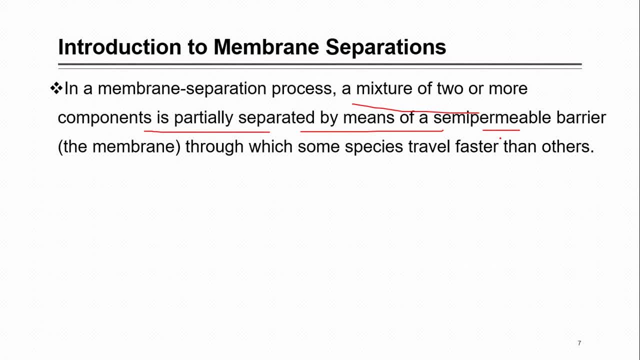 like 1 of the salt. you know that there are various salts present in the water. for example, there can be NaCl, MgCl2, mean and some other like KCl, and I mean it will depend on from where you are taking the water, So there can be as well some other chemicals present. 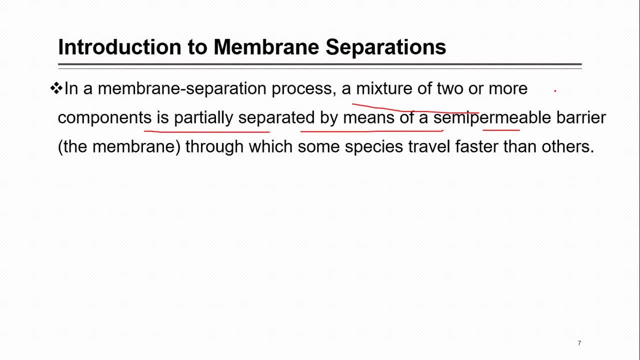 inside this, for example, you can say organic hydrocarbons are present, So there can be more than 2 components but this membrane which we are going to use. actually, this will be selective for some of those component. it will not reject or it will. 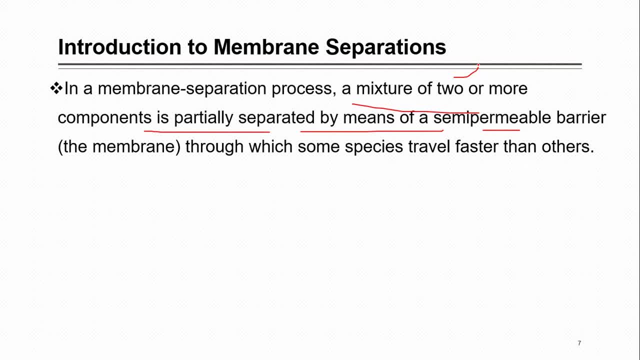 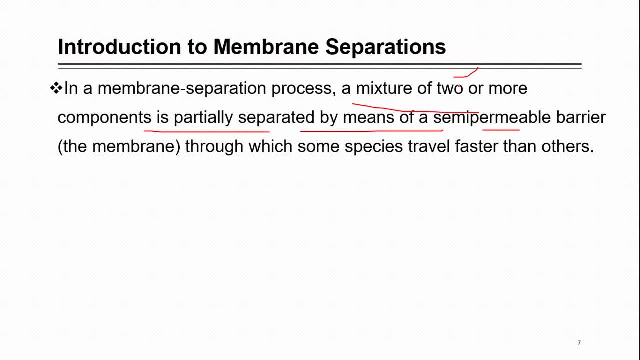 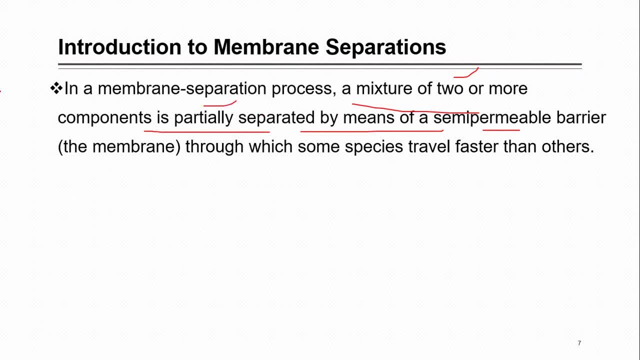 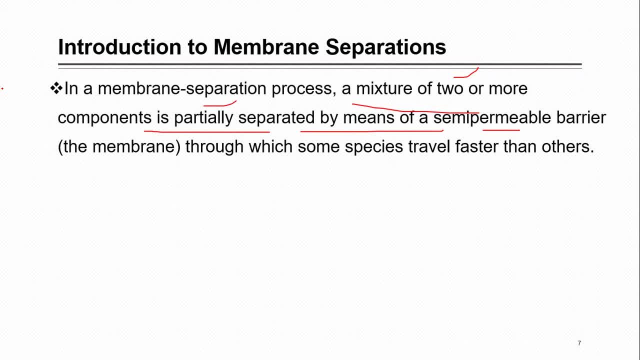 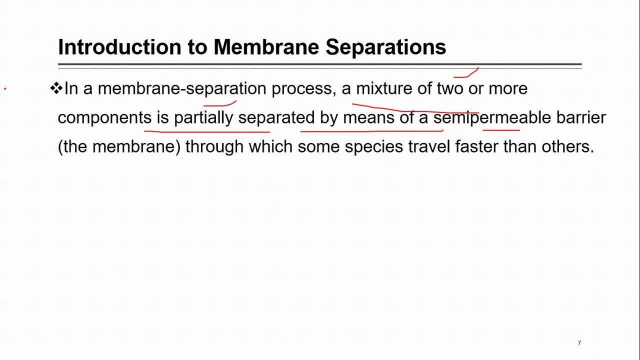 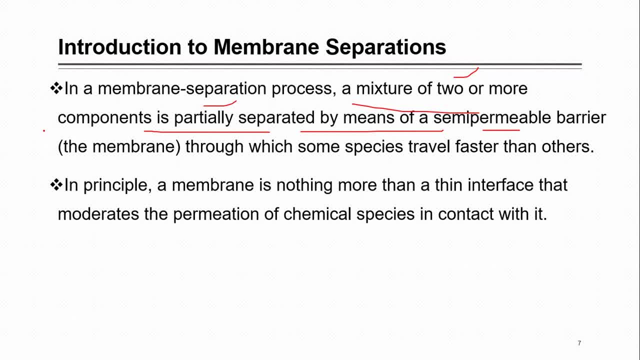 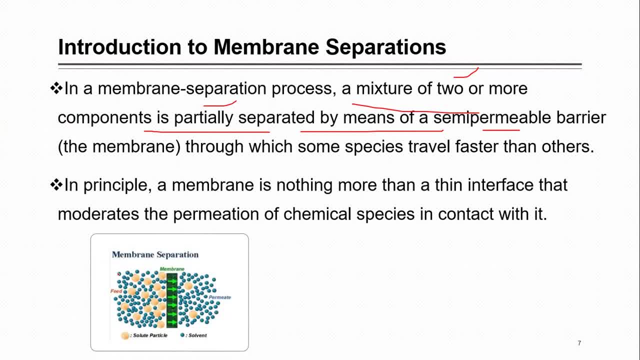 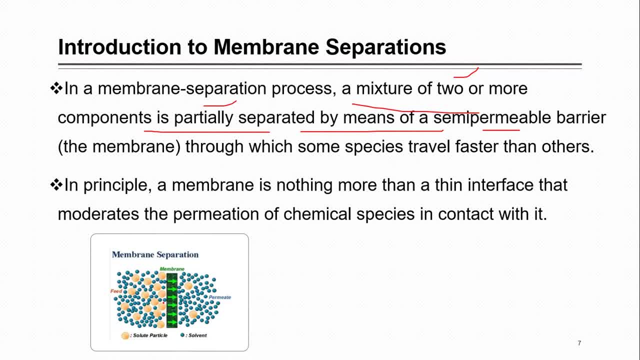 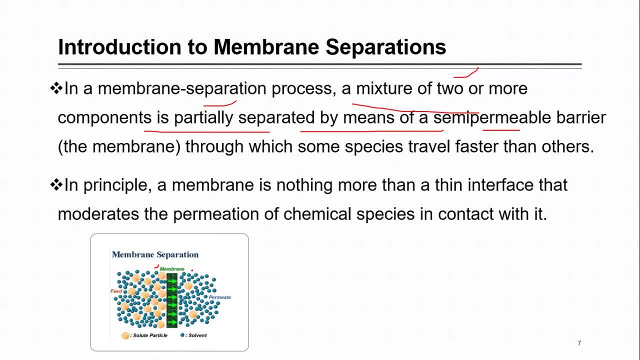 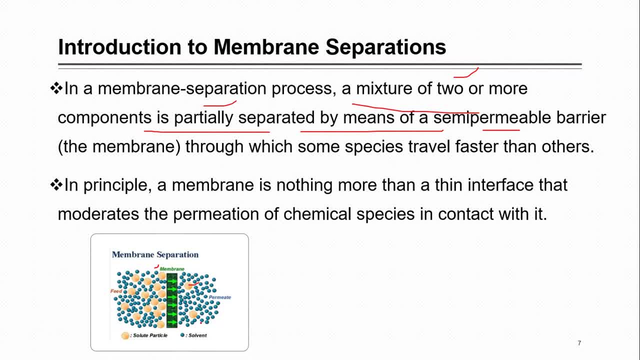 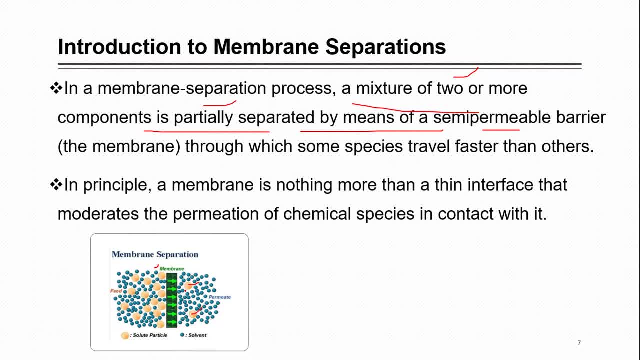 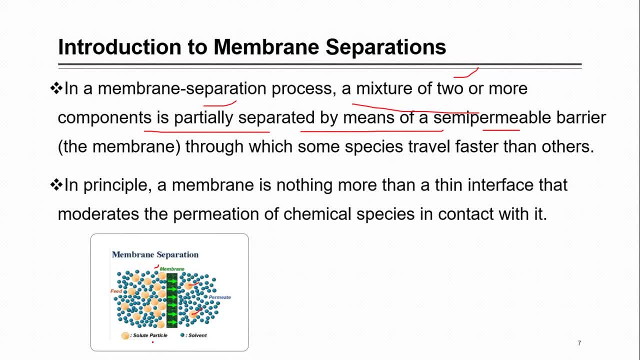 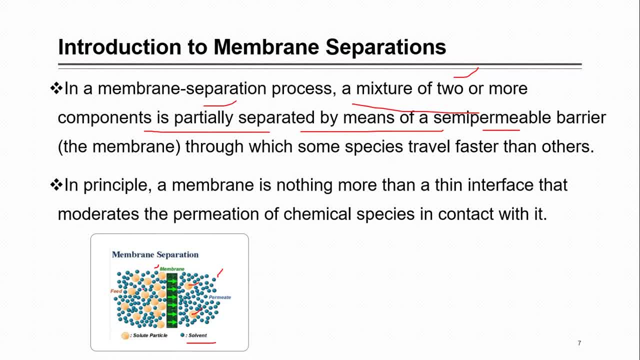 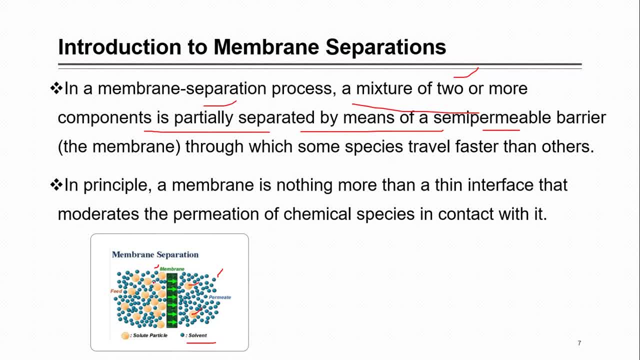 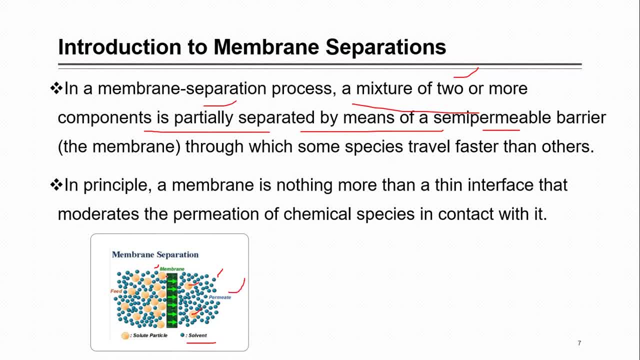 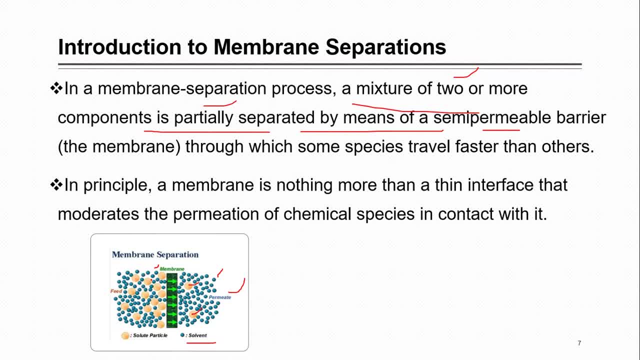 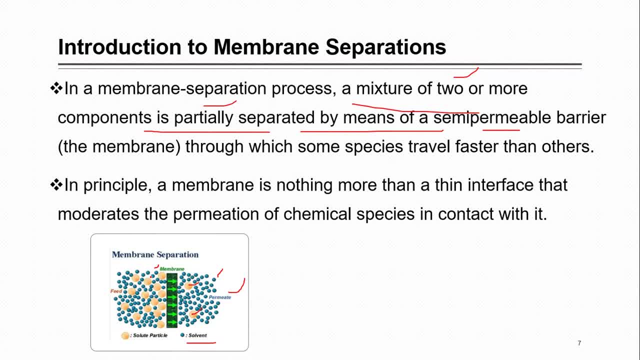 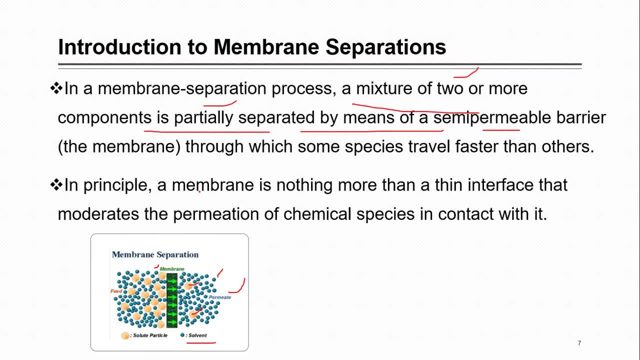 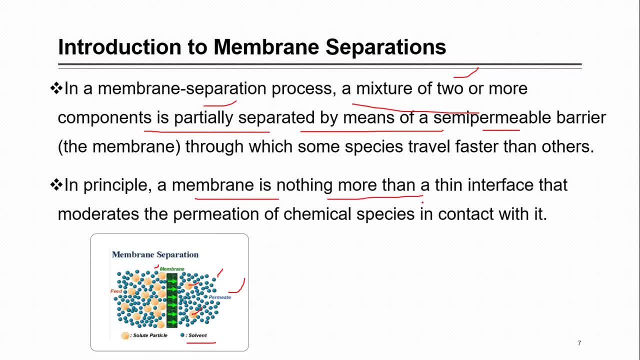 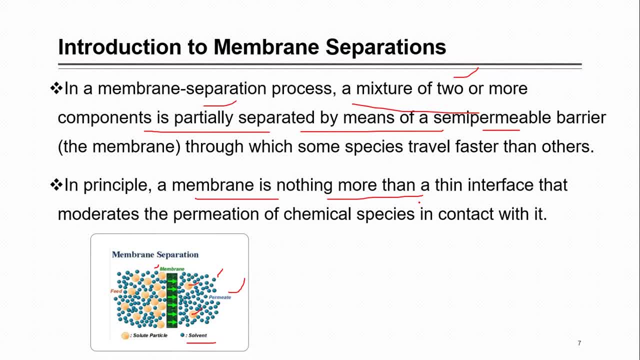 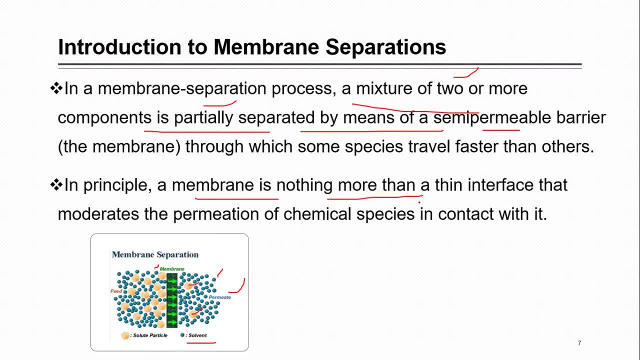 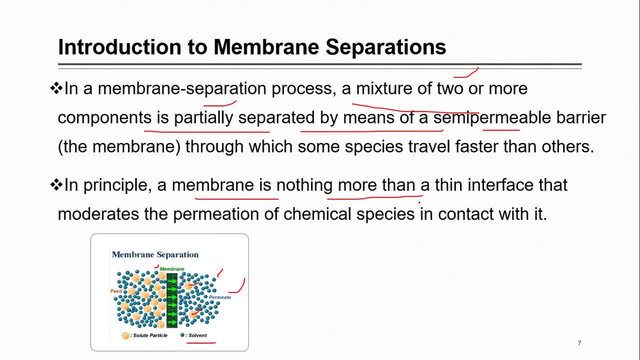 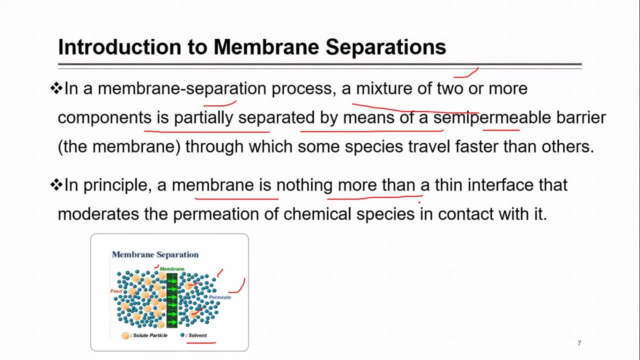 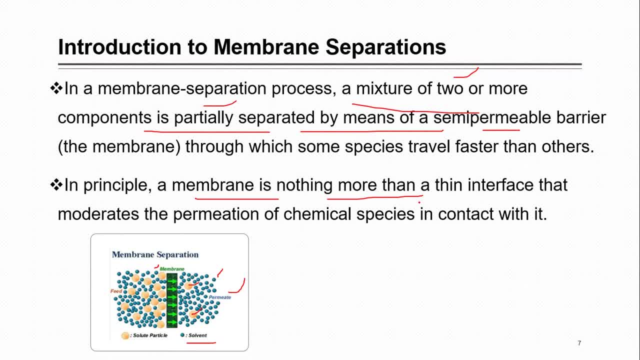 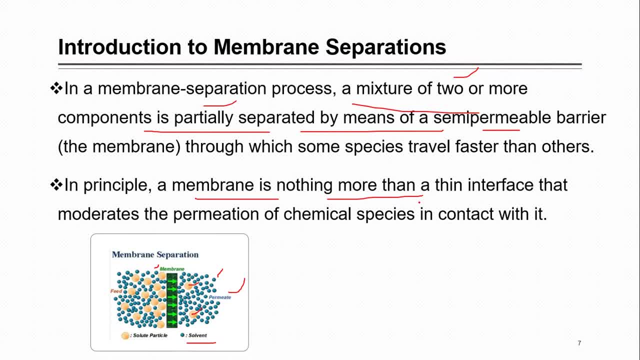 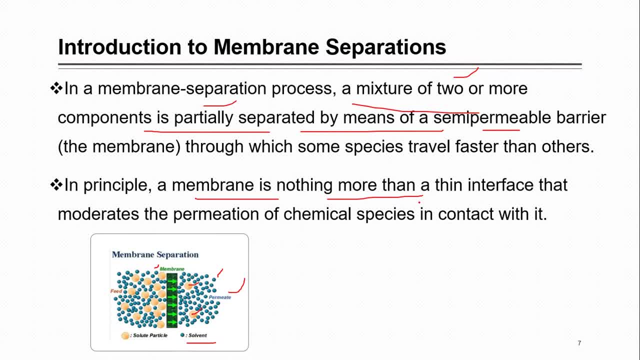 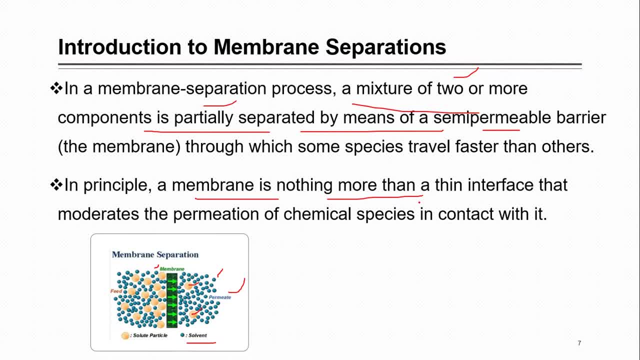 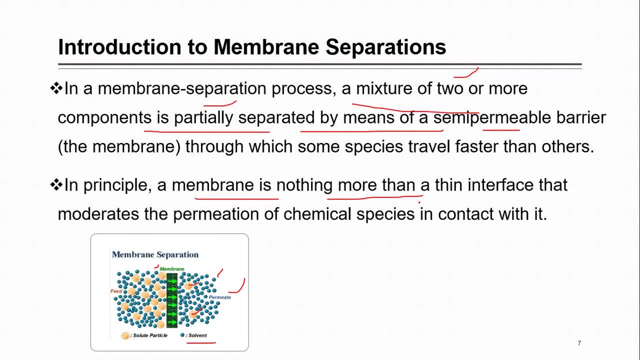 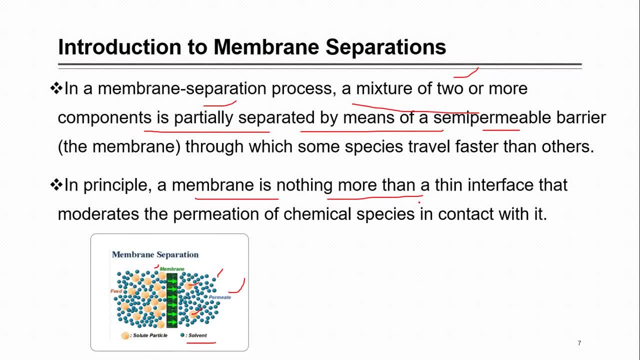 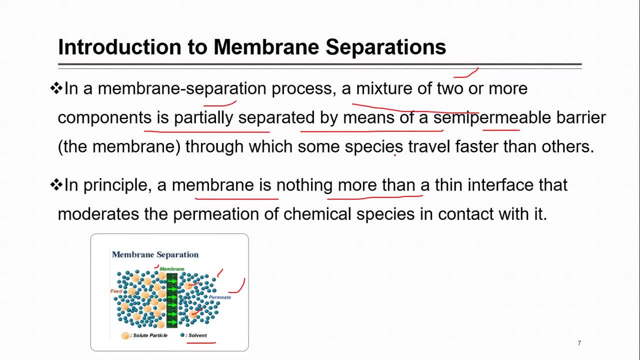 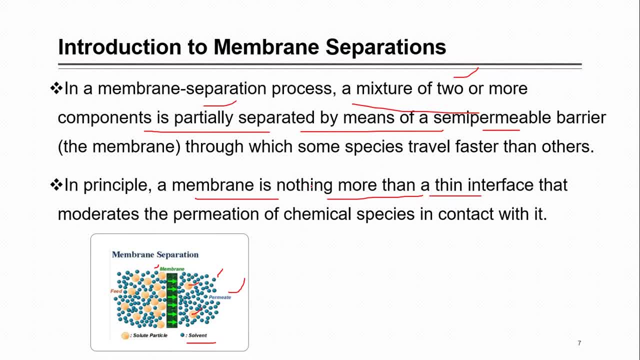 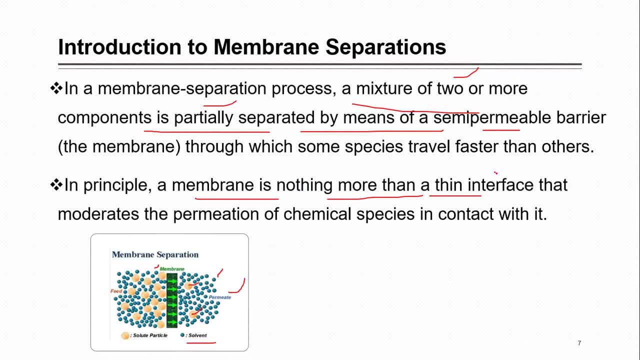 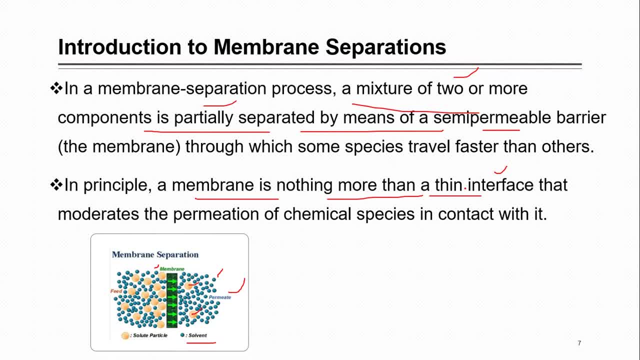 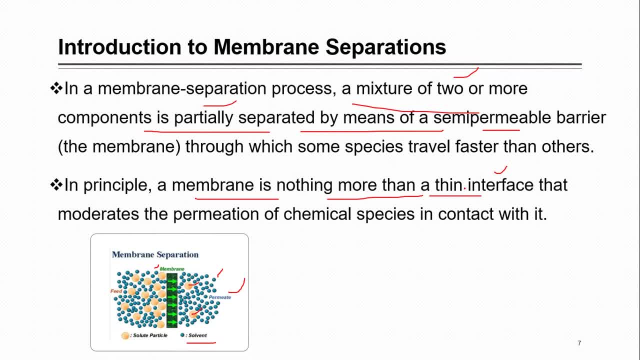 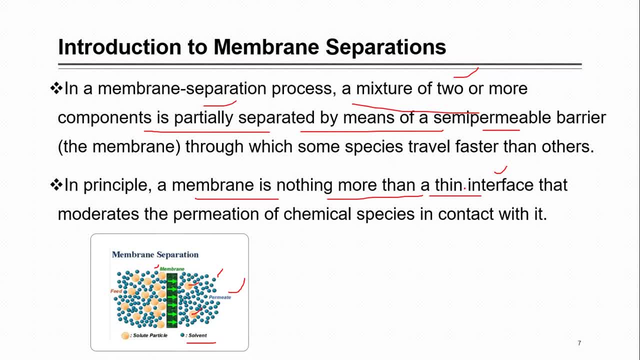 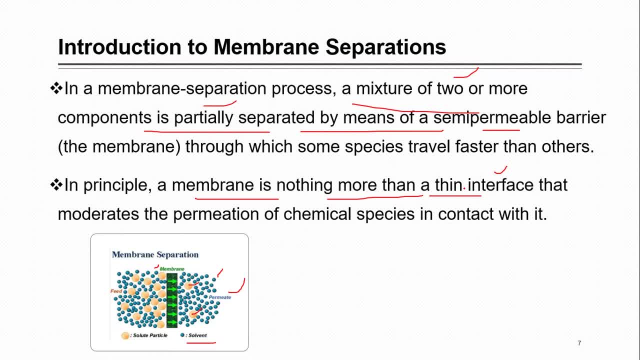 So to remove various component, or if you can have more than 1.. So to remove various component, or if you can have more than 1.. that there is a interface. interface is actually in liquid-liquid extraction when we were talking about this. 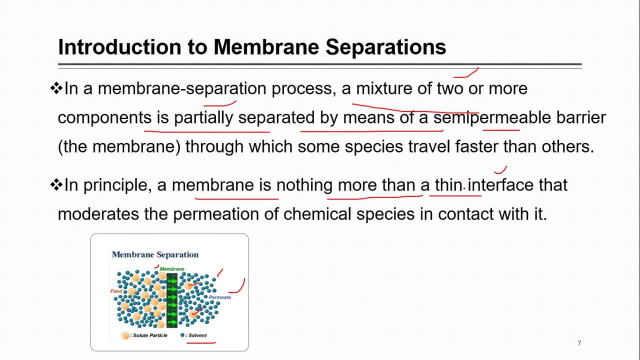 So that is means some two of those components are coming in contact with each other, as we were bringing our feed and solvent in contact with each other. So some interface. there will be some boundary actually where their contact is taking place. So here this is thin interface through which actually separation is taking place that moderates. 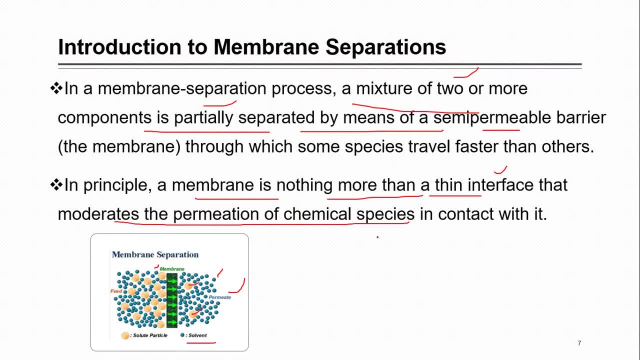 the permeation of chemical species in contact with it. So permeation, this is from permeate, so that allows or that moderates the passage of some chemical species which are coming in contact with this. suppose here we have somehow the similar example: some feed is moving through this. you will look at this membrane later. 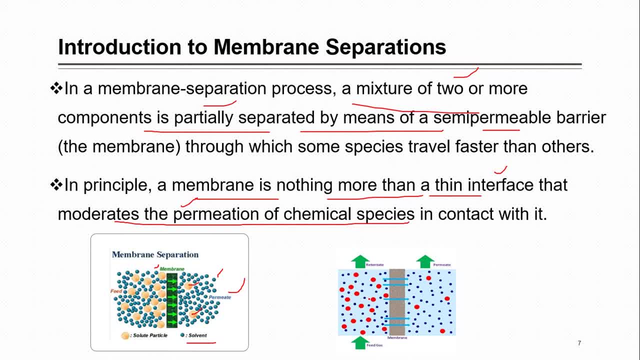 like there are various type of setup or assemblies through which we can pass our feed and get it separated. So, overall, some of those component, while this feed is passing through this in this direction, so some of those component will travel or will pass through- will permeate through this. 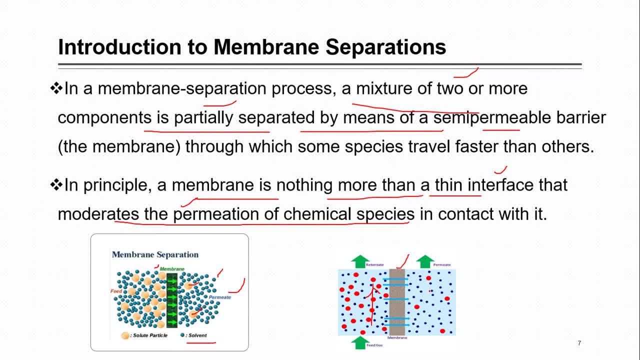 membrane. this is membrane barrier, So they will go on the opposite side and that is called then permeate, because something which has passed through the membrane is straight named as permeate, and while other which are not passed through this and they are still left as such when it is leaving this system. 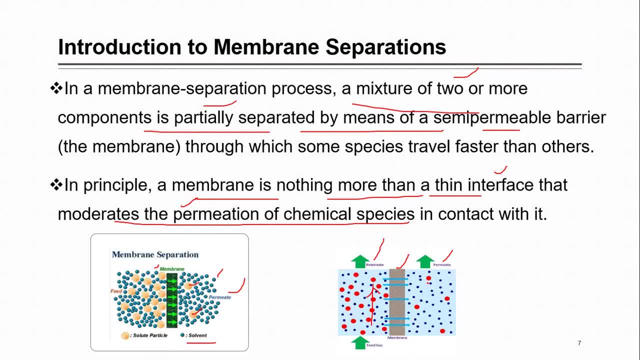 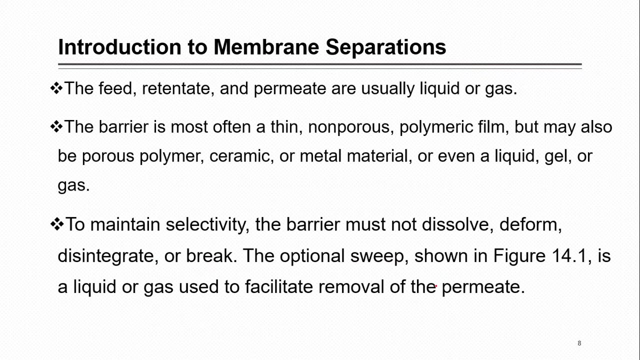 so that is called retintate And 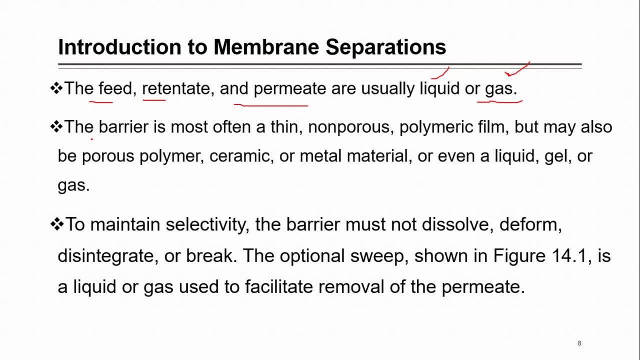 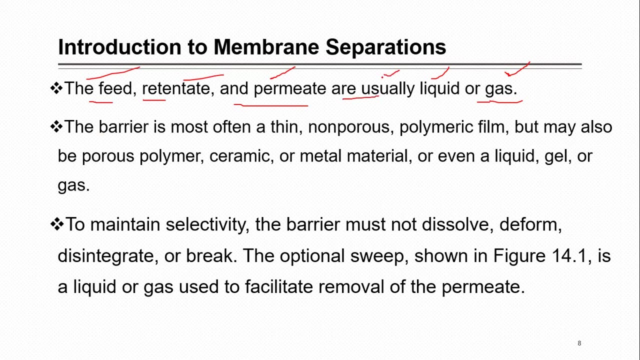 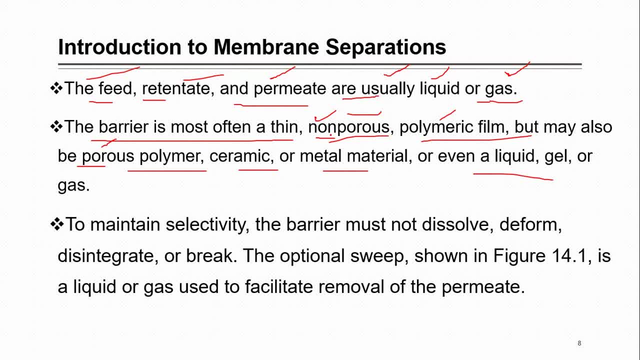 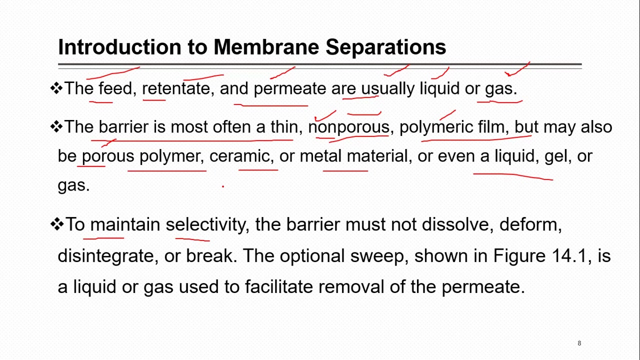 When you look at these membrane and we are looking for specific selectivity. selectivity mean I mean something which we want to selectively remove with the help of this, So to maintain selectively. barrier must not dissolve, deform, disintegrate or break. It means actually your. 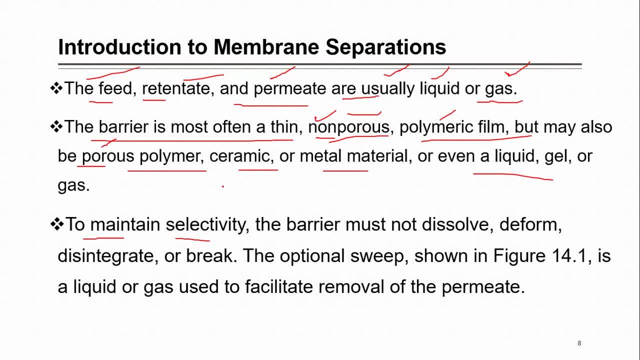 membrane should be stable. it should not be like a reactive. it should not dissolve inside your feed. I mean it should not break. if it will break, definitely, I mean this will not be working properly as well if it dissolve some of its component or remove with the feed. 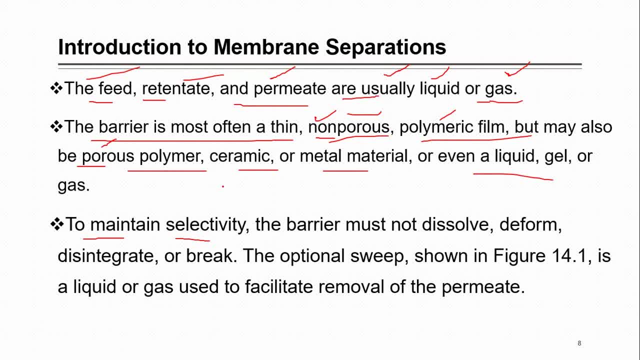 they become part of the feed in the form of retentate or permeate, So that will be actually the damage. So in order to avoid that, mean that membrane: if you want purity, you want good separation, So your membrane should not have like these kind of problems. 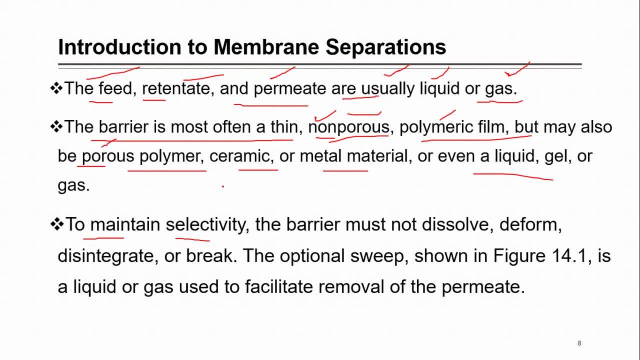 Like optional sweep which we have seen somewhere inside the figure which I have told you that this is from your text book. So optional sweep we were using that was being used to facilitate removal of the permeate. So I mean we have seen at this at that time I have 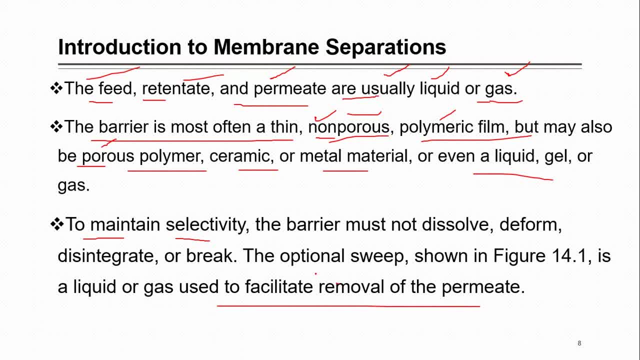 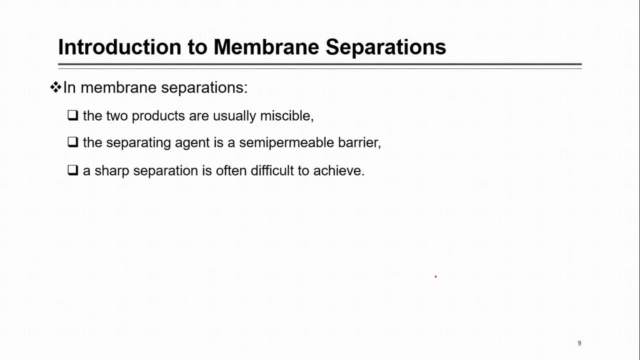 told you that you can just pass some liquid gas through this system at the high pressure So that it will push the permeate which is accumulated inside system. that can be easily removed. So overall, when you look at these membrane separation, actually I mean the products which 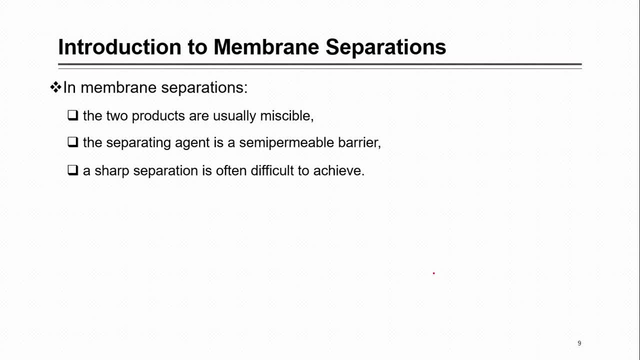 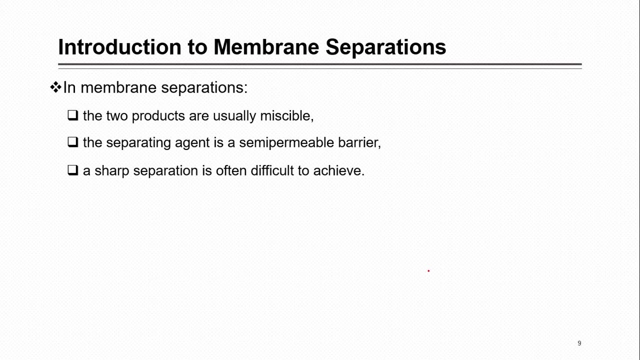 you are getting here in the from the feed. they are usually miscible, Like. what does this mean? I mean they are usually soluble. I mean in the form of one phase, For example. I mean here we have talked about one thing like 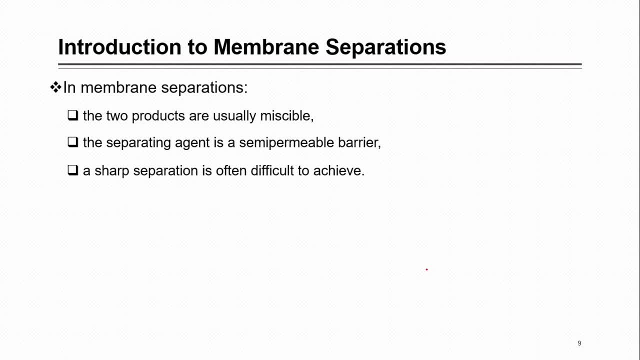 gas, natural gas and natural gases in the form of like mixture of gases, So they all are miscible with each other. They will be, they will appear in the form of one phase actually. I mean you cannot distinguish between them. So when you will pass through this membrane, 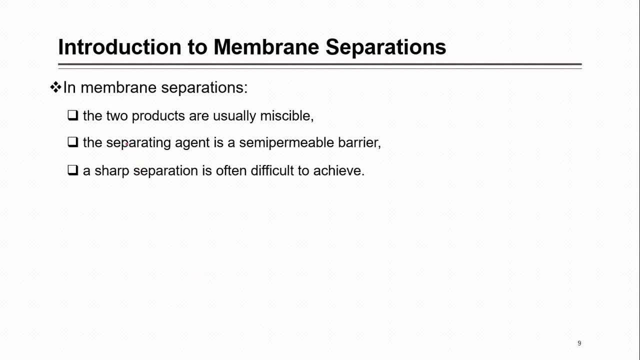 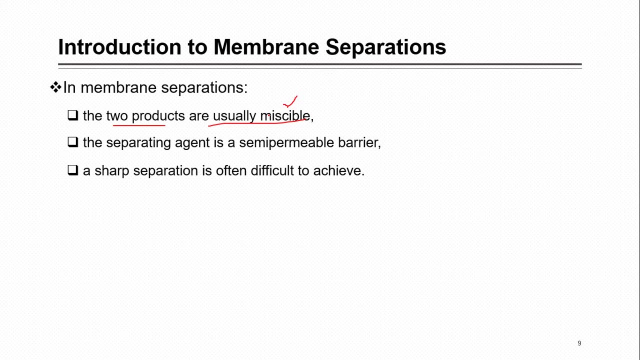 the products which you are getting. they are now separated, like one is permeate and other is retentate, But initially they were the two products which you are getting in the form of permeate and retentate. they were miscible. I mean when they are miscible. so this the problem. 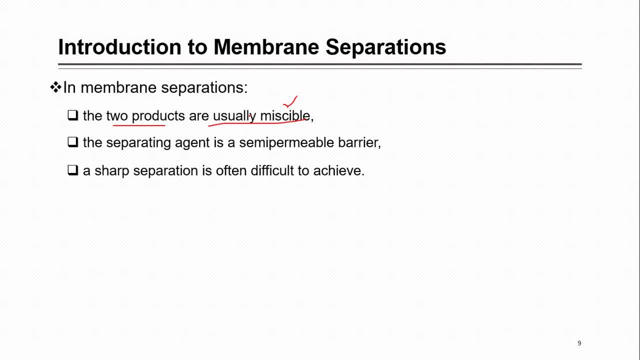 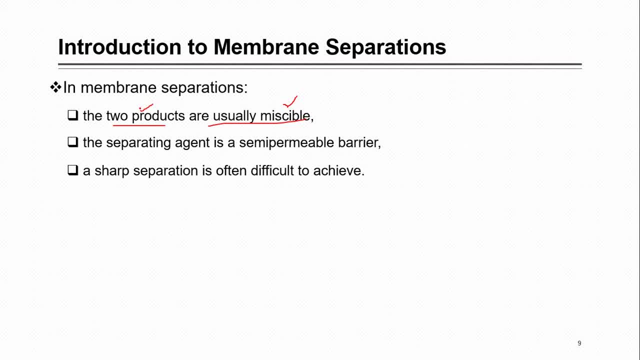 So they can be separated with this membrane into two component, and then they will be like just separated out. They will become somehow we can say immiscible, not immiscible in terms of this separation. Actually they will get separated. The separating agent here is: 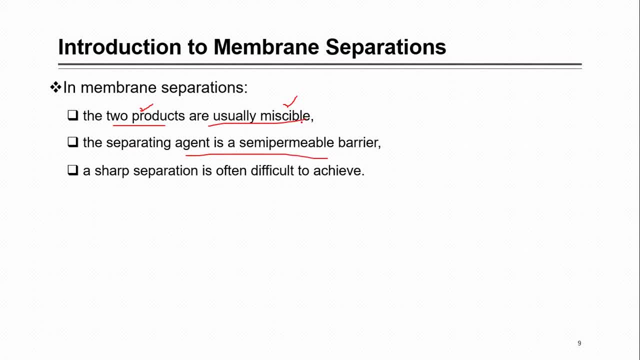 semi-permeable barrier. Actually, when you just compare this technique with the other techniques which you have talked about, So you can see that separating agent. always we look at some separating agent, like if you are looking at phase creation separation, So in which the phase 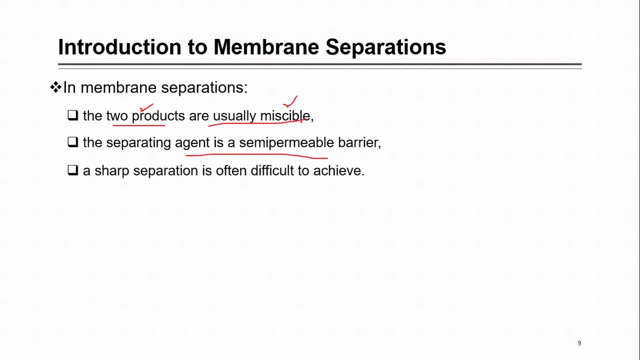 is created with the help of like may be temperature or pressure, as we have seen, some cold drink. So when you open the lid, so what happens? actually? you are reducing the pressure. So here your pressure is the separating agent as well. if, in distillation, you heat the feed, So there the heat. 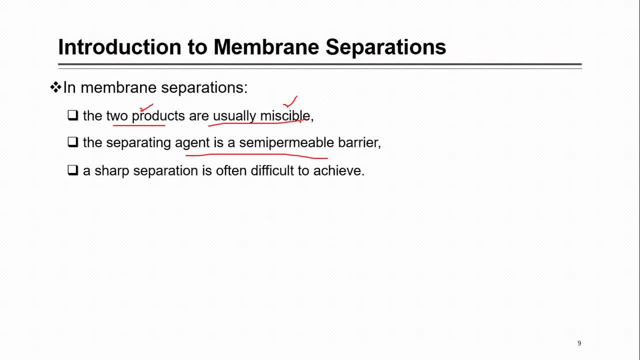 the temperature is your separating agent. In liquid-liquid extraction you have to separate the liquid. There are some parts of the liquid that are separated out. So here in distillation you have seen that our externally introduced liquid was the separating agent. Inside absorption. 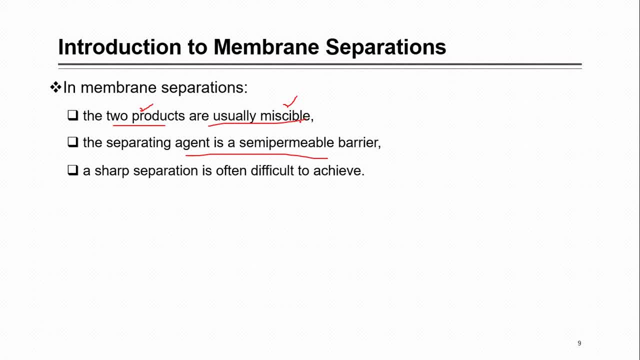 you remember that some externally introduced solvent which was absorbing some of the component through the main feed, that was separating agent. So here actually separating agent is some semi-permeable barrier and that is membrane. So here in membrane separation, sharp separation is often difficult. Sharp separation has 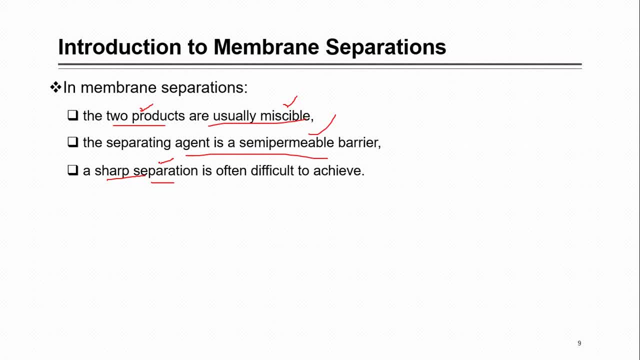 we have seen sharp separation mean, mean, as you have seen, that 100 percent separation. I mean that is a bit difficult because membrane will allow some of the components- other component will also to pass through, which we do not want actually mean they are not like 100 percent. 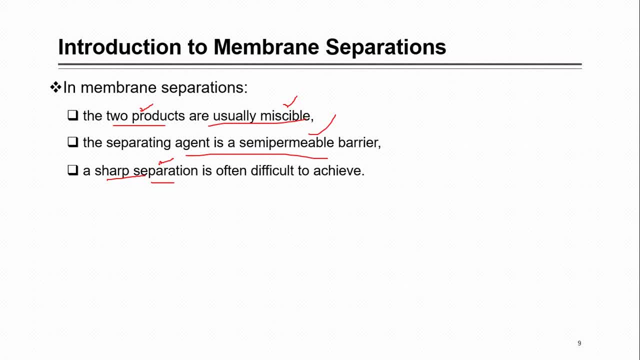 removing, and this problem exist in more or less all techniques. actually, you cannot get 100 percent separation, or if you are looking for very high purity or such stuff, may you go for more than one stage. is that we also talked about this, like in liquid, liquid extraction as well mean? 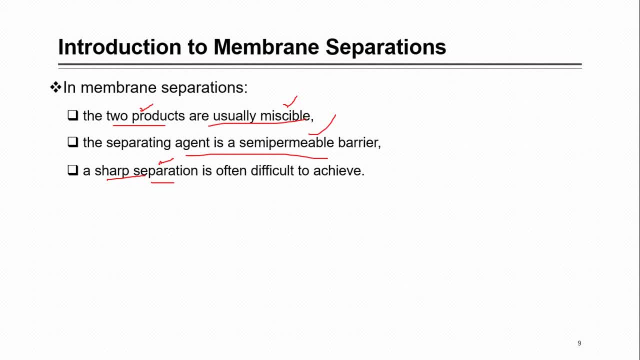 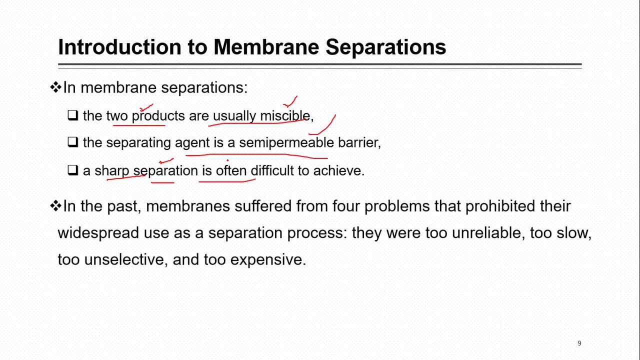 in absorption or distillation, you know that we have more than one stages. so again here in membrane separation, due to this we can have some time more than one stages are more than one module to pass and your feed through this that you can get better separation. so when we look at the membranes, actually they are being used in industries now many industries. 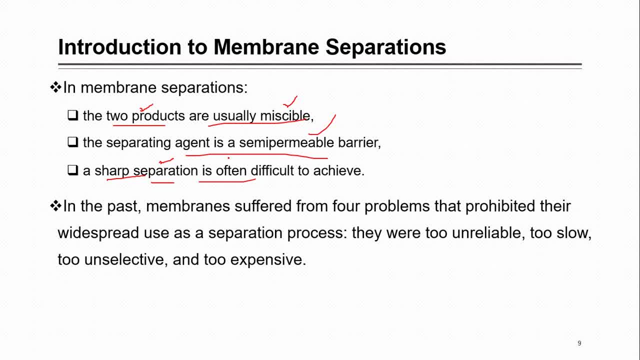 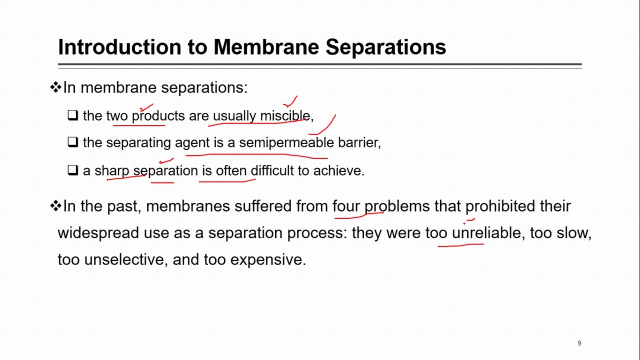 are using these membranes on commercial scale mean they are being used. but if we look at the past, actually mean membrane has suffered from various problem and they were actually four common problems which membrane were facing, and those include actually they were too unreliable to unreliable mean they were not giving very good separation: sometime they are performing well, sometime they are not. 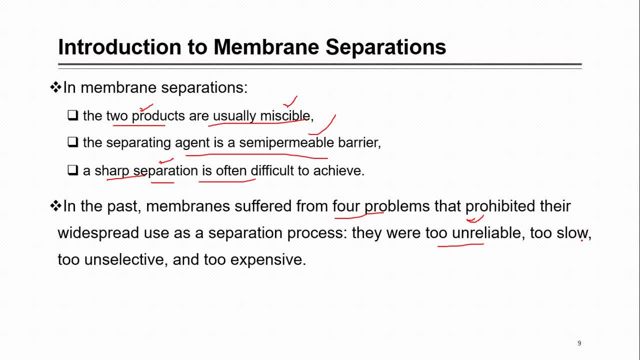 as well. they have some problems like they were too slow, because this is the barrier, as we have seen, that if membrane is sometime porous, sometime non-porous membrane can be used. so if you are using, like some of non-porous, definitely mean there are no pores and now you have to separate. 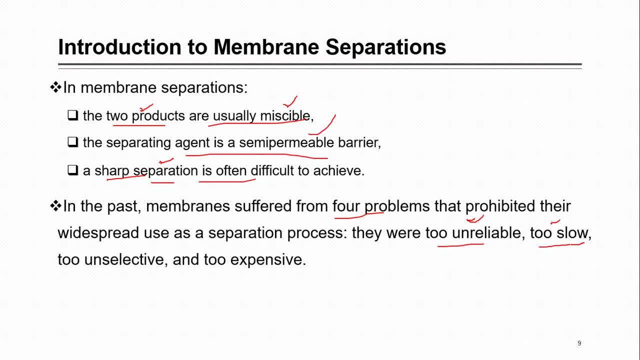 two components, so it works somehow like slowly as well. you can have like they are too select, unselective, because when we want to separate the feed, suppose we were separating natural gas, CH4, from the impurities, CO2 or H2S. so it is like it allows along with. 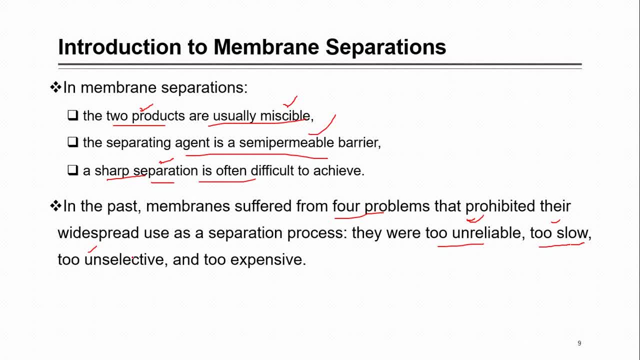 natural gas, CH4 and other hydrocarbon. it allows also CO2 plus H2S to pass through. or for example, you can take the example of air if we want to separate it into oxygen and nitrogen. so I mean, if you allow air to pass through this membrane and suppose we just consider that this 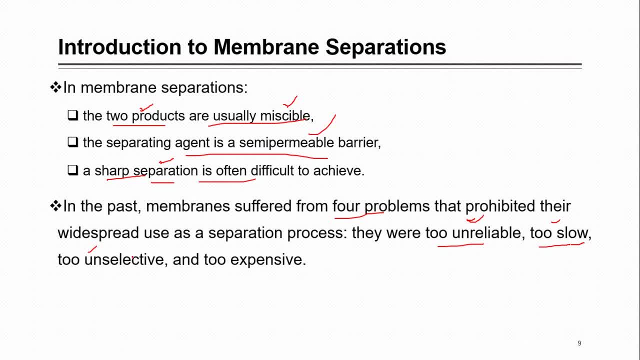 is selective towards oxygen. selective towards oxygen mean it allows oxygen to pass through mainly, but with this some nitrogen will also pass through this system, so that is become mean that make it like unselective. that is, allowing other component which we were looking to be separated that also pass through this. so this was a problem of unselectivity and they. 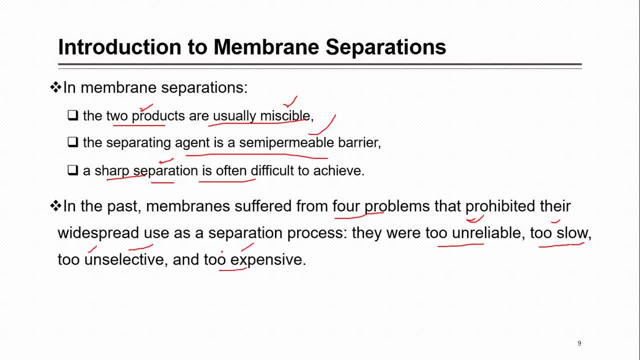 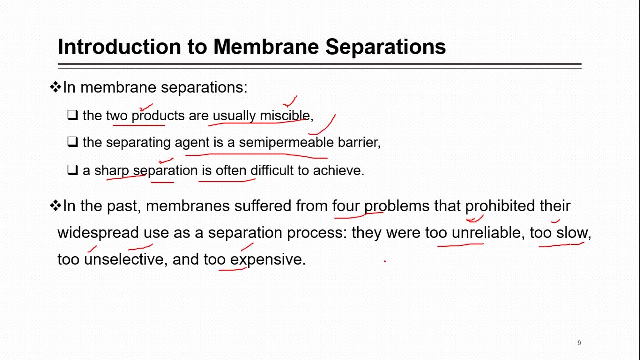 were also too expensive mean it is expensive to build the system. so when you have compared these main membranes with the other technology, the existing system, like distillation, absorption and liquid extraction or some other techniques, so compared to them these four problems were present in membranes but with the passage of time in these problem has been. 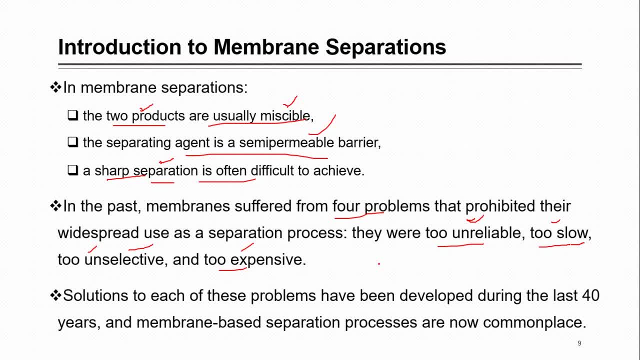 solved in the last 40 years or so, more or less more you can see, I think, book reference 爸爸. so based on that, actually the membranes have been developed and their performance has become better. so they are being commonly used in the industries now. so here is a brief history. 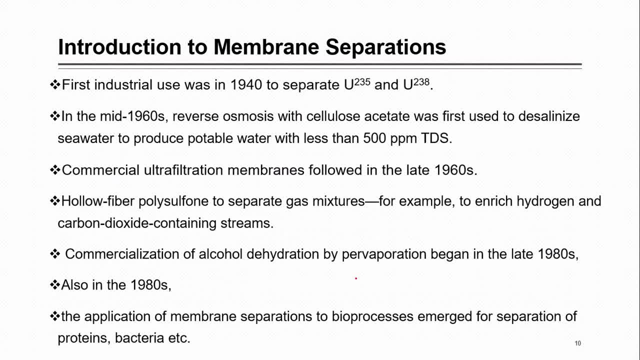 of the membranes. for when you look at the membranes, so where they have been used and when they have been used, so you can see that because of this condition, a certain memory as a selectłem into rate, they cannot be terminated totally prior. no change date after the rested membrane they go through, which nuclear process also takes a time, like cost and stress, where membrane through films which must be legible in any cell vessel setting. 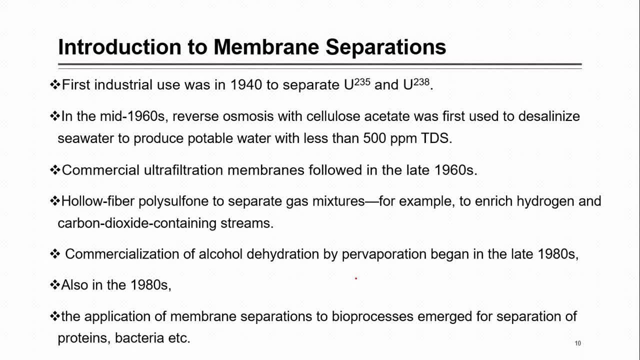 otheraker is a discarding its own product is considered a self help from top. madam, their first industrial use of the membrane was in like 1940 and that was used for separation of uranium components. that was in the form of uranium fluoride, I think, and you have separated. 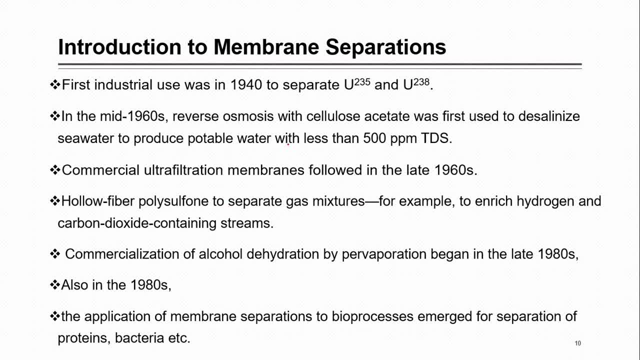 two isotopes of uranium through this. So here you can see this 1940. what is important about this year? So if you remember, this is the time of World War II and at that time mostly you will look here. there is also another main year in which actually the most of somehow. 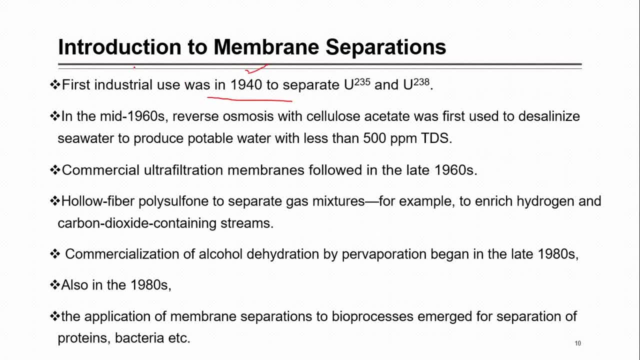 development took place. So in that time this industrial use of this membrane took place, and that is the time when the first industrial use of the membrane took place. So in that you have separated uranium isotopes with the help of membrane, So that was first industrial. 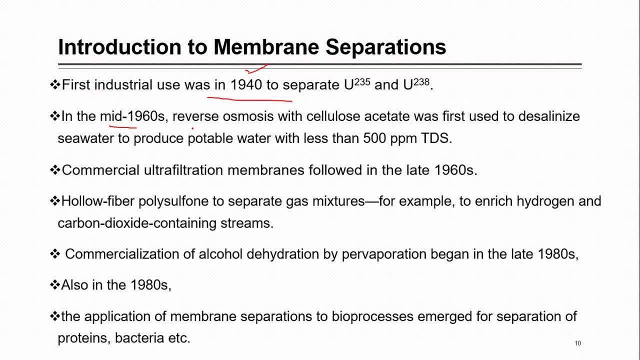 use of membrane and then, like in mid 1960, reverse osmosis with the cellulose acetate. I mean reverse osmosis is one of the membrane separation technique which we have to discuss in detail. So, in that you have used cellulose acetate, 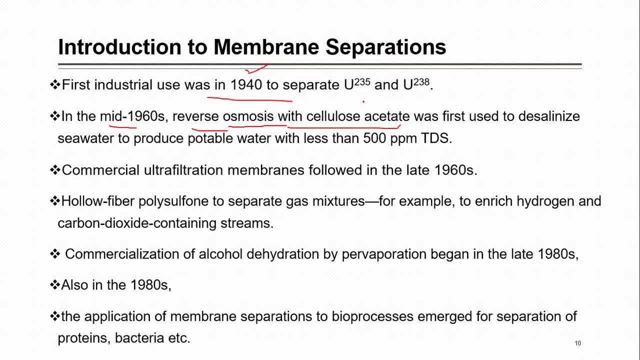 membrane. Now cellulose acetate is actually material of construction of those membrane. reverse osmosis is the phenomena in which you have used cellulose acetate membrane, and they were used first time in the mid 1960. they were used for purification of sea water. 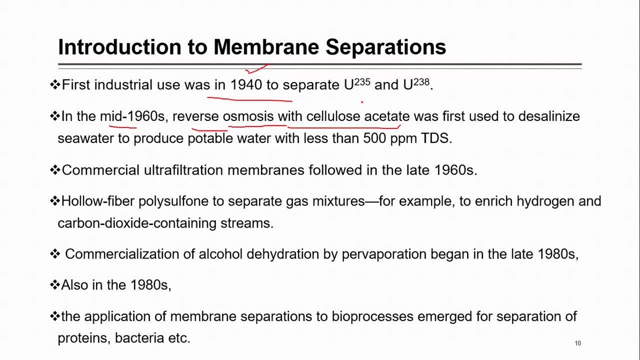 So it becomes available or means suitable for drinking purpose. and the first time- here I mean from this sea water solids were reduced to like 500 ppm. TDS means total dissolved solids. So they were reduced to less than 500 ppm and with the help of this, when they are less. 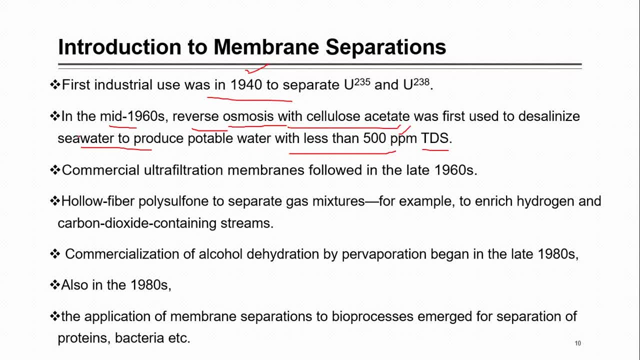 than 500. usually this water is drinkable, but actually in sea water, if you look at the sea water, So that contains very high amount of these total dissolved solid. they are somehow in the range of, I think, 30000 ppm to 50000 ppm mostly. 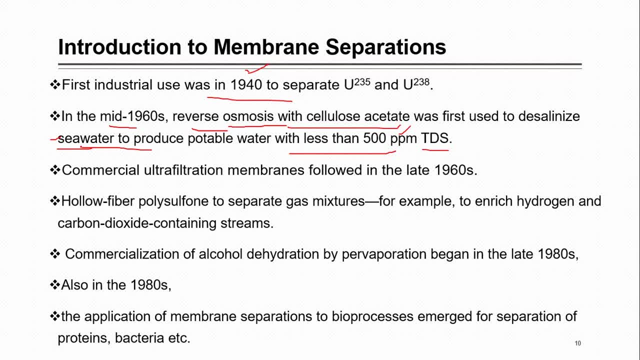 So they are reduced to high. you can see here that now at these membrane reduced those from the 30,000, or somehow mean they, this is very big value, So to say 500 ppm. So this was first industrial use of cellulose acetate for cleaning of water, sea water. 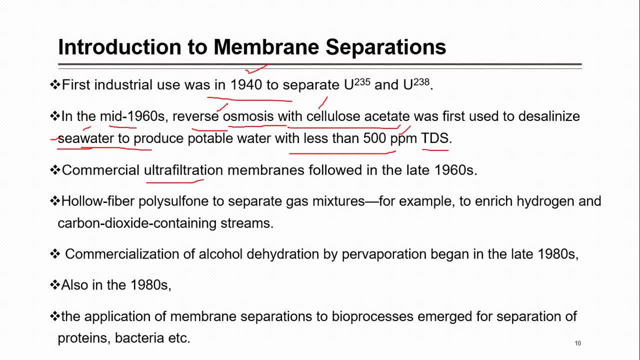 Then there is one type of membrane. ultrafiltration like this is also one type reverse osmosis. So ultrafiltration, this is based on actually their size, pore size ultrafiltration. then you will hear, I think see something called microfiltration, somewhere may be mentioned. 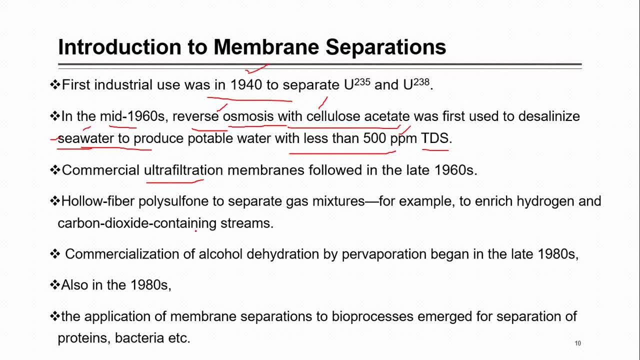 or that. that is also one type. So ultrafiltration was also followed in like 1960 after this reverse osmosis- somehow that was also used on industrial scale, mean, that membrane was also used. Then there were hollow fiber polysulfone, membrane polysulfone, now again one of the polymer mean. 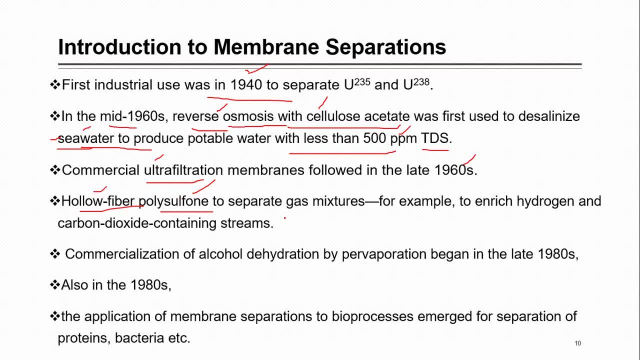 with the help of that, some these hollow fiber membranes were formed and they were used for separating the gas mixture first time, So that gas mixture was actually hydrogen and CO 2 mixture, So that this membrane were used for their enriching or their mean separation. 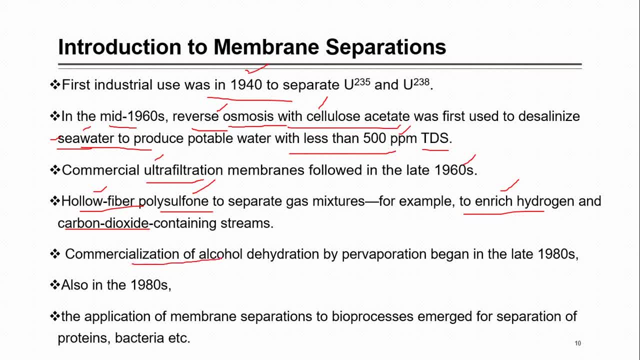 And then their mean commercial commercialization of alcohol dehydration by per vaporization. a per vaporization is one of the technique in membrane. again, we will talk about this in detail later on. So this is the part of main. they study this chapter. So in that actually also here we actually, but we do alcohol dehydration. what does this? 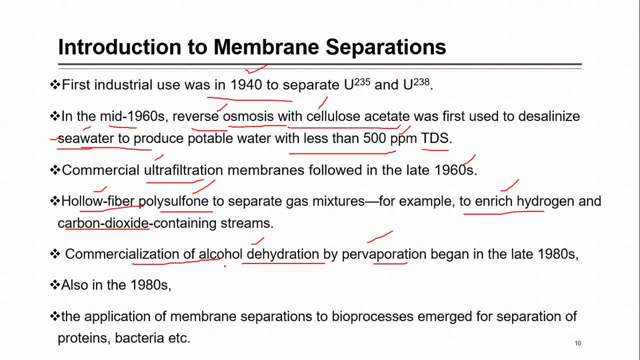 mean like removal of water from alcohol, So through per vaporization. So, overall, you can see, you will see, in this technique actually we have a membrane as well. here vaporization is taking place. So based on this, we have a per vaporizationnamed it as per vaporization. 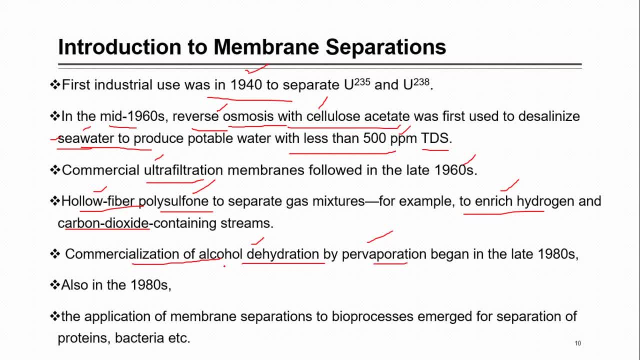 we remove the water so through this technique, and that took place in white. like late 1980s, also in 1980s the application of membrane separation to bio processes took place and if you will look at the literature, mean in this era. 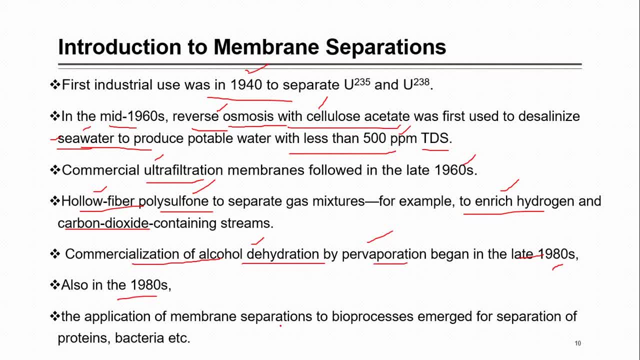 also a lot of development took place and I think it was the time of, like Arab Israel war, I think, and in that time many developments took place. so like they were also used for bio processes and in bio processing, actually, what you do, you separate the some high proteins. they were also used for the separation, or 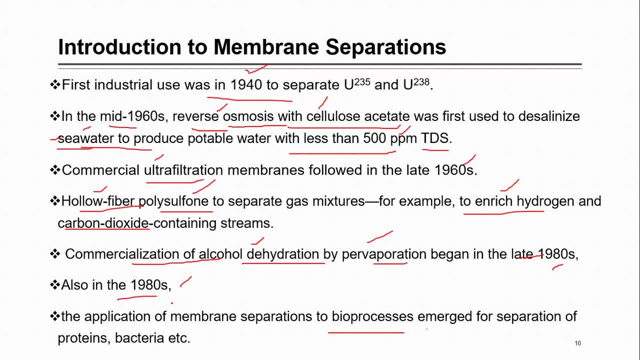 main separation of bacteria and yeast, somehow. so this is this brief introduction about membrane separation in terms of like their development with the passage of time. so, as I said here there is some terminology like ultra filtration, there is pervaporation, there is reverse osmosis and I was talking about also micro filtration. so 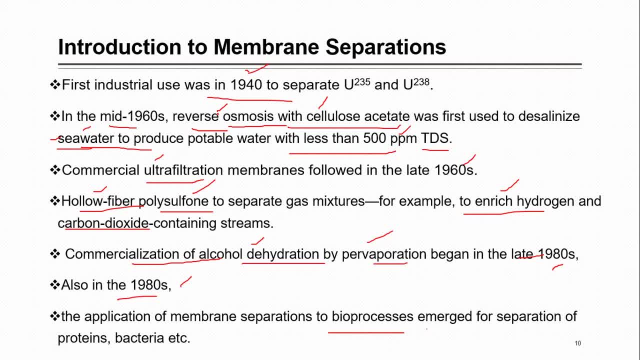 don't worry about these. these we have to define later on. I mean just because this is introductory lecture and some of the terminologies will not be clear to you, but we will talk about them in detail, actually, later on. so but just from here, remember that they were developed. you know that with the passage of time, 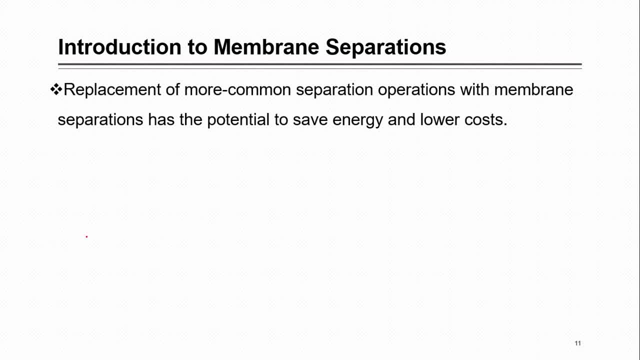 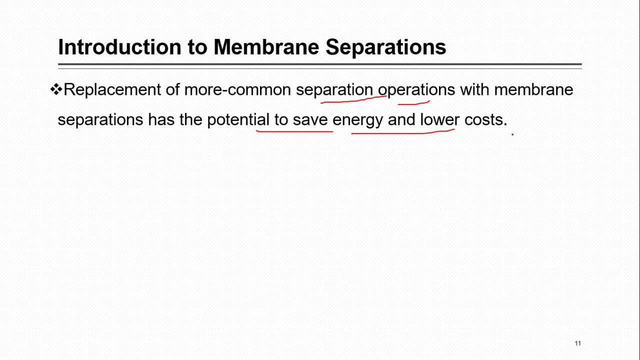 so if we want to replace other- I mean separation operation with the membrane, so they that can be beneficial to save energy as well as with in terms of cost. actually, once, like back, we talked about this that in the initial stages membrane were not like reliable, they were slow, they were expensive. but with the passage, 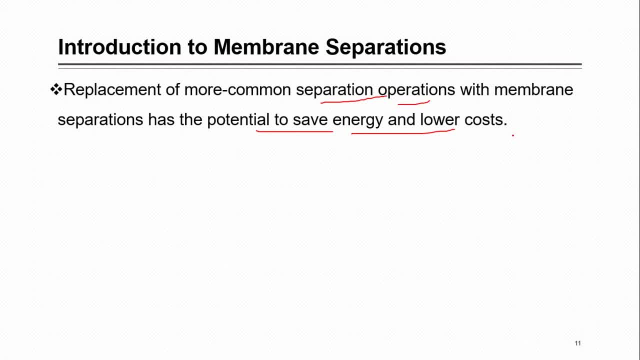 of time. many improvements has taken place as well. their price has reduced and they have been reduced so people can get. they were super different models. the difference went between different points of any wisdom. so was it that slow they were explained? 357.". revise: will they have become more reliable due to this? they are being used on industrial scale, but still. 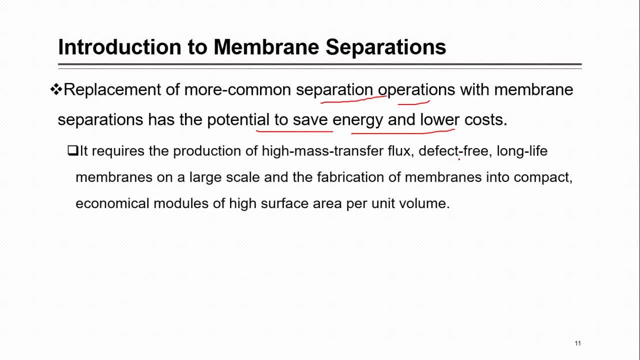 I mean there are some problem, like they require high mass transfer flux. mass transfer flux mean actually, as we said, that we have to pass components through the membrane. so they should provide good flux based on selectivity, like they should be selective for one component and they should allow, I mean, good mass transfer of that component through the membrane as well. 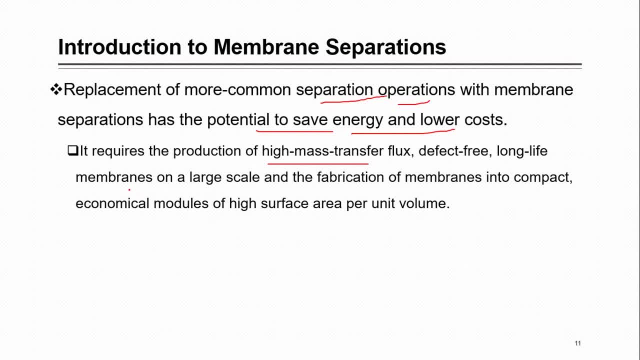 they should be defect free and long life membrane on the large scale. I mean these are some requirements like they should be defect free, they should be, they should have long life, because if you will study the membrane you will see that most of the time membrane still in the industry is you. 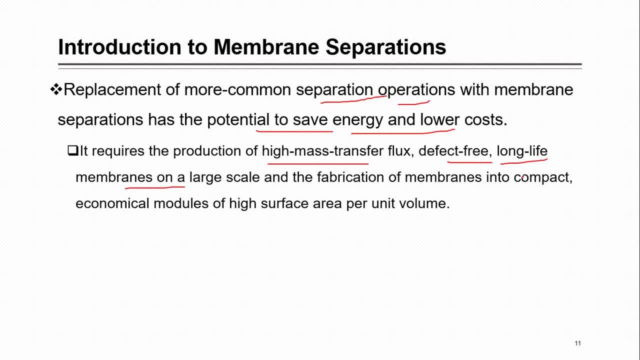 have to replace the membrane, maybe after one or two year at some time, it depends on the application, maybe after a few months. so that's the problem, if you are. I mean just replacing membrane after every few months, So that will become expensive process. So if we can design such membranes which provide good 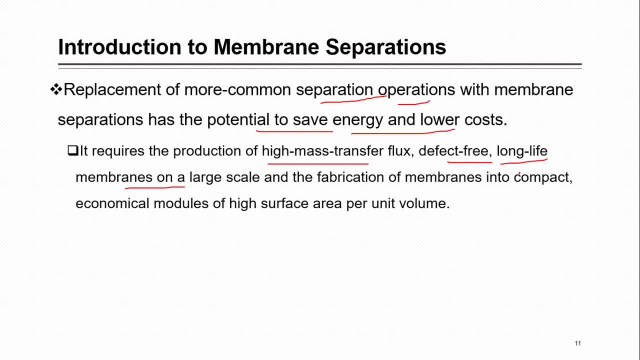 flex and they are also long lasting, so that can be good replacement of other separation processes on large scale as well. the other requirement is like we should have, I mean, build this membrane module into the compact and their fabrication should be compact. Compact mean actually they should have high surface area per unit volume. 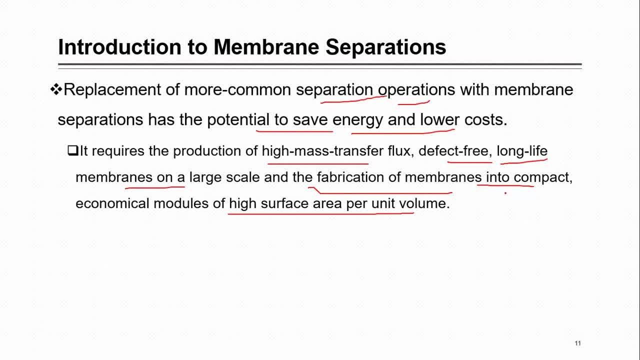 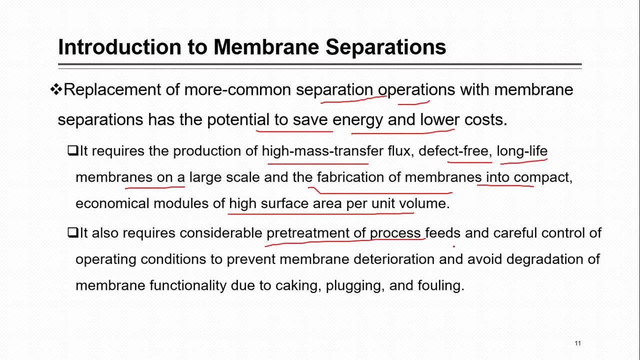 So they occupy less space and overall their construction is easy. So these then can be. it can be advantageous as compared to the other separation technique which are commonly used in the industries. At the same time, this replacement also requires something considerable: pretreatment of the process feed. What does this mean, actually, when you pass some components through the membrane? 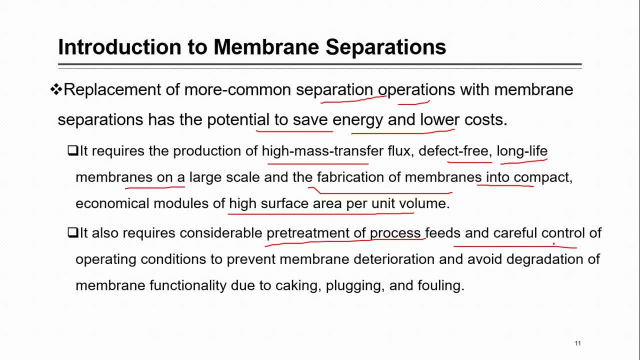 you are looking for the separation through the membrane. Sometime cake formation can occur. So the separation cake mean one layer of the cake take place on the surface of membrane. I can give you the example here: like in the lab, like we have seen lab scale, separation through the funnel mean you are passing your solution and that is separated into like I mean solid and the liquid. 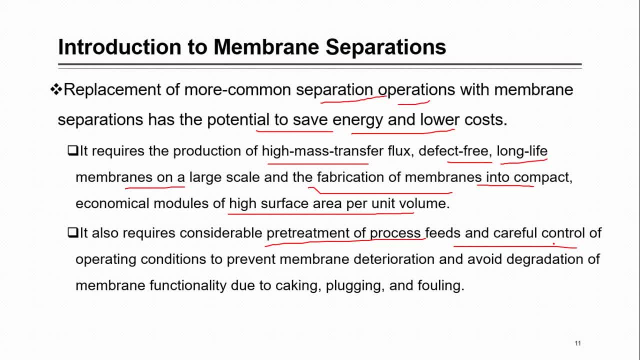 So the solid which is left over on the surface of filter, what you call it cake. those crystals are named as cake actually. So that same can take place on the surface of membrane when you are passing Some of those component through the membrane. So, if like, look at the water containing. 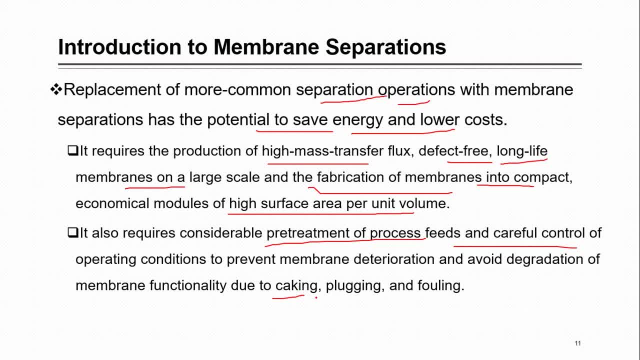 salt, So water pass through And if salts are retained on the surface they can form cake there and that cake can actually plug and as well foul the surface of that membrane. So membrane should be such that it did not allow these cake formation as well as plugging and fouling. 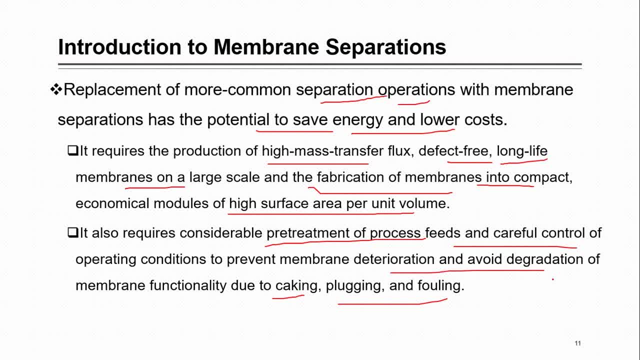 Because if this takes place, this will definitely deteriorate and degrade the quality as well. it will create difficulty in the separation because if some cake is formed on the surface of membrane, maybe you will need now more pressure to pass your liquid through this, So that will add on operational cost. So in order to avoid those problem, membranes are being designed in such a way that these problem can be minimized. I mean, you cannot eliminate them, but you can reduce them. 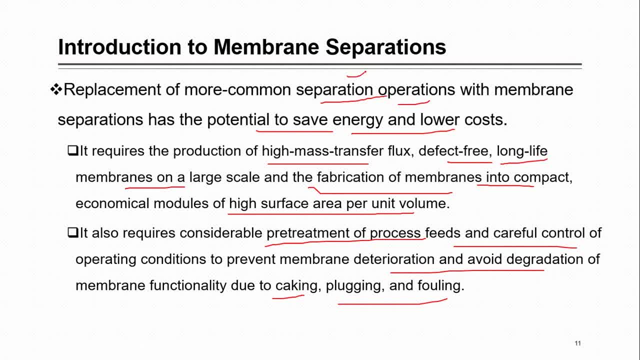 So these are some requirements which can help us to replace all other separation processes with these membrane, If we can design some membrane which allow good selectivity, good flex as well. they are long lasting, they can be compact and they did not allow the formation of these plugs or cakes on its surface. 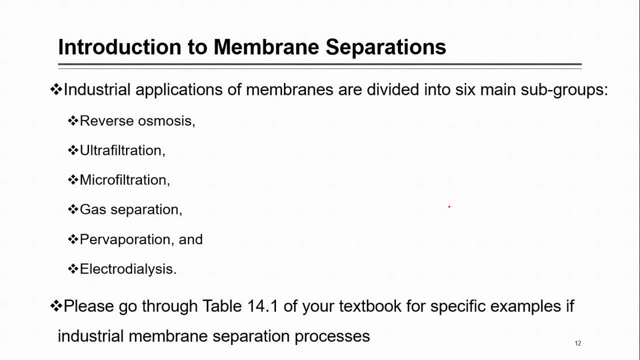 So overall, when we look at the industrial application of membranes, So they can be used in many ways, So they can be divided actually into the six subgroups and those subgroup include: like there is reverse osmosis, then ultrafiltration, microfiltration, then there is gas separation, pervaporation and then electrodialysis. 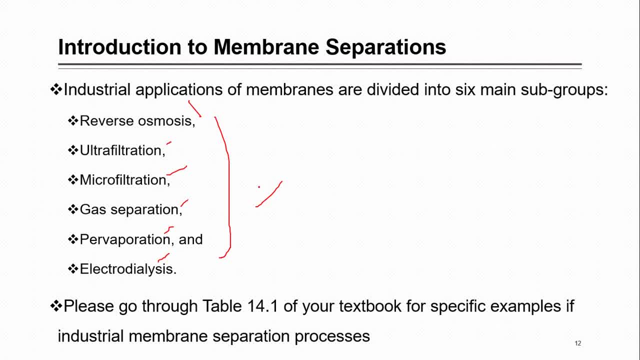 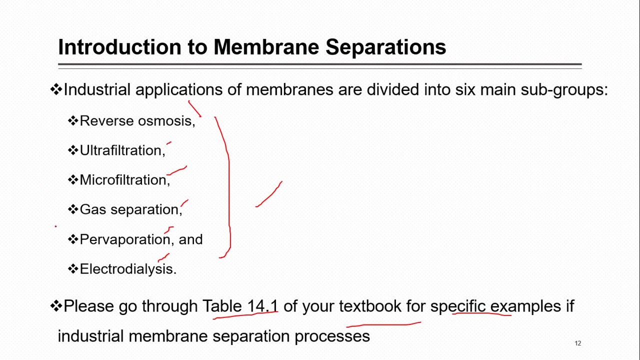 And actually all these are used for some specific application. So kindly go through the table 14.1 of your textbook and there you will see specific industrial example for all of these main categories. You will see that they are being used for some specific application. All of those He has provided us various example that this is used for this purpose, this purpose and so on. So overall, like, for example, if we say gas separation, so that's used for like natural gas separation as well, where there are various other examples of its industrial application. So reverse osmosis, that is used for usually water cleaning in the form of, like maybe water, ground water. 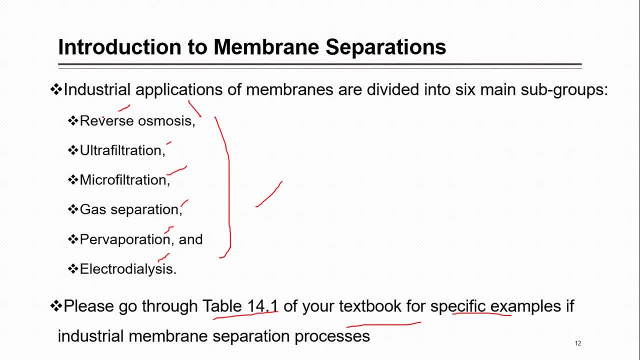 Even cleaning as well, like sea water. So many other you will look at, I mean for all of these techniques. So kindly go through that table and just remember few of those, For example. at least you should remember one of one or two for each of these techniques. 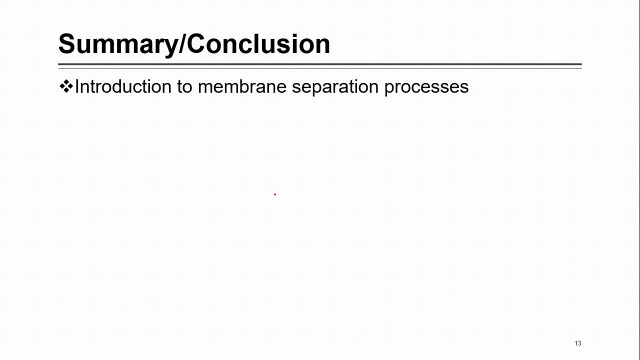 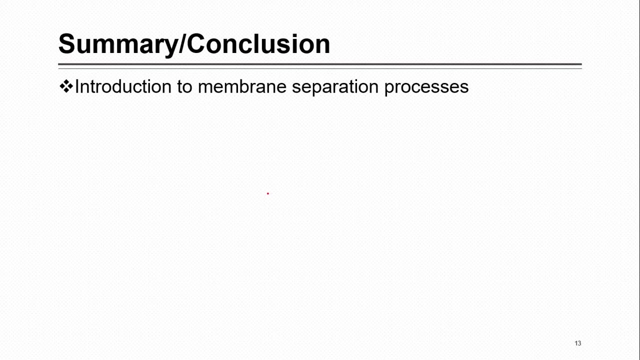 So that's it up to here. actually, today I have introduced you only with the separation through the barrier, and membrane is one of those barrier. Actually, we started with the very common example which we have discussed earlier in the semester, in the start, So through those were actually usually the filters, like water filter. There is filter inside lab which you use. 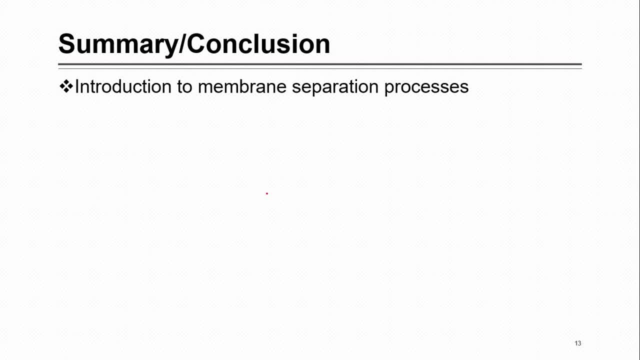 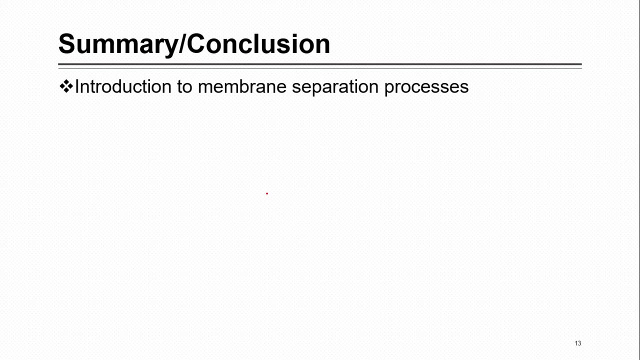 as well. There were air filters, some oil filters, So then we jump towards membrane. So membrane are also a barrier, but they are- I mean, working in a bit different way- like they can be porous, they can be non-porous. Most of the filter, when you see, filters are actually porous, But membranes can be porous as well as non-porous. So here size based separation, as well as some other phenomena, like based on diffusion separation, can take place. 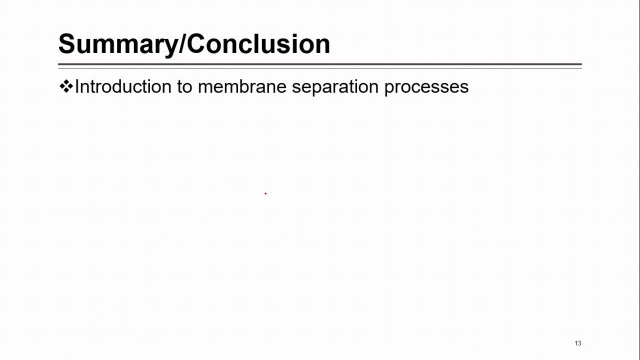 So then we have generally look at this, that when you are separating the feed through the membrane, that is separated in retentate and permeate. We have defined those and also we have looked at some of the industrial example when membrane started developing and some of the problem with membrane phase still facing. So then at the end we have seen that membrane application are actually divided into the six categories on industrial scale And they are, I mean, they have different names actually they have different application And then from here, inshallah, we will continue in the next class. Thank you, 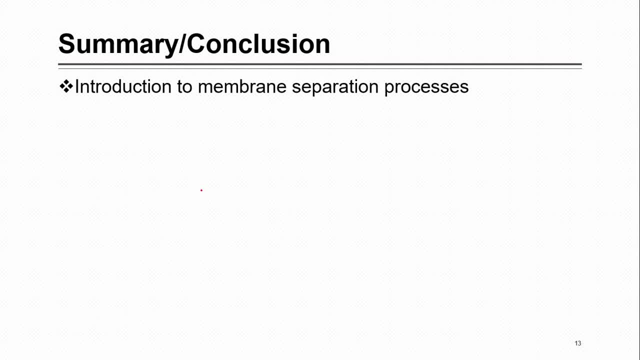 lecture about this industrial application. Thank you so much.